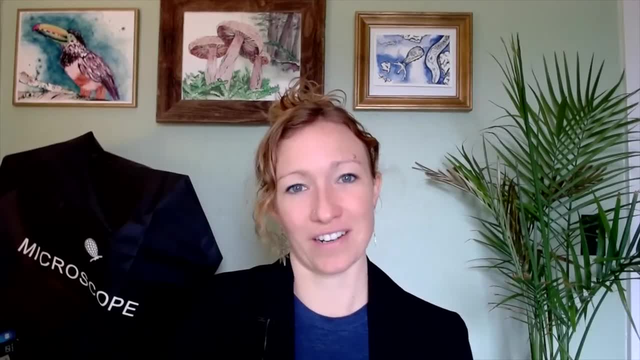 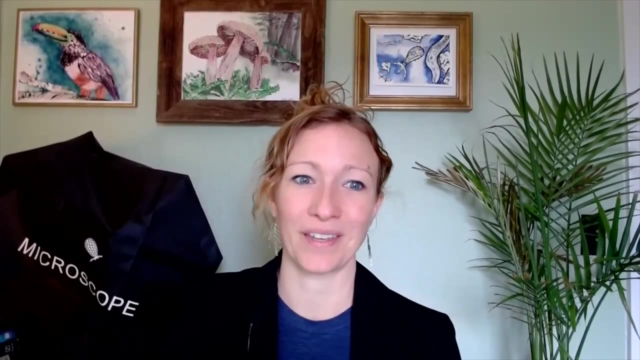 run local trained organization of farmers in the deep bed farming methods, So I am so thrilled to be a part of this that supports TNEE and their work. So thank you for everything you're out there doing TNEE farmers. Today we get to zoom in on the interactions between organisms in the soil. 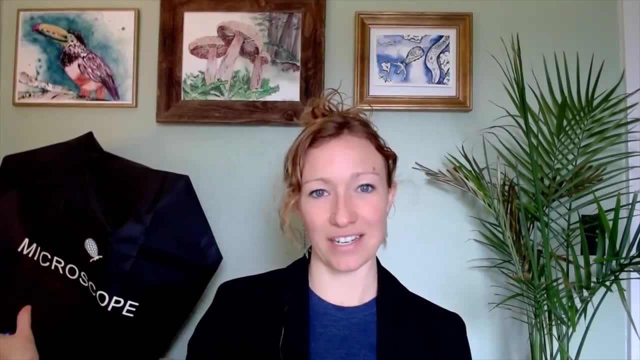 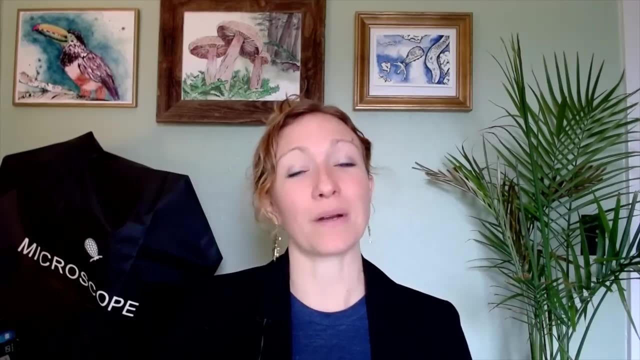 and zoom out to landscape level ecology. in our science day We will kick off the science behind the scenes of TNEE. So let's get started. TNEE is a program designed regenerative agriculture with Dr Mary Cole, plant pathologist. 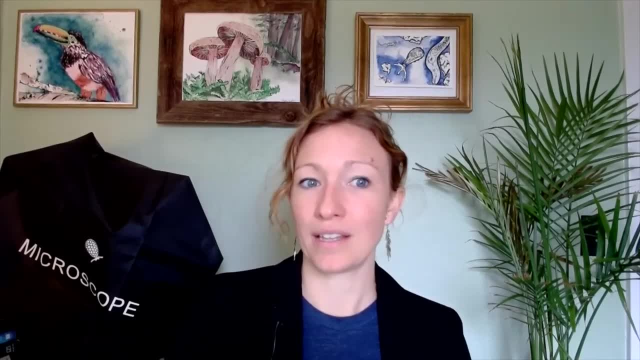 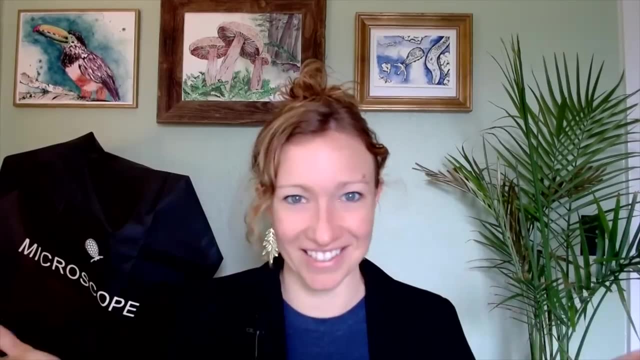 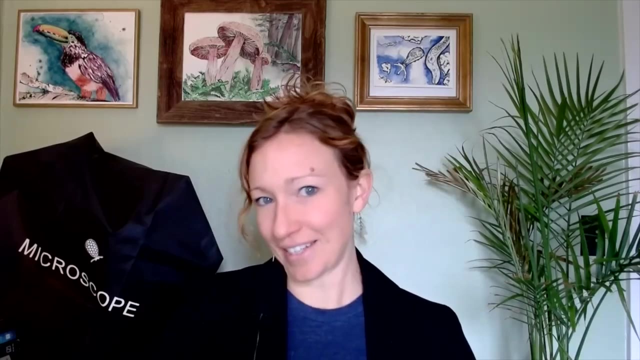 soil microbiologist and the founder of AgPath. We have Dr Christina Young, a dryland ecologist and founder of Science Moab, And then I get to give a talk today, if you haven't heard enough from me already. I will talk more about plant insect interactions and the role of the soil. 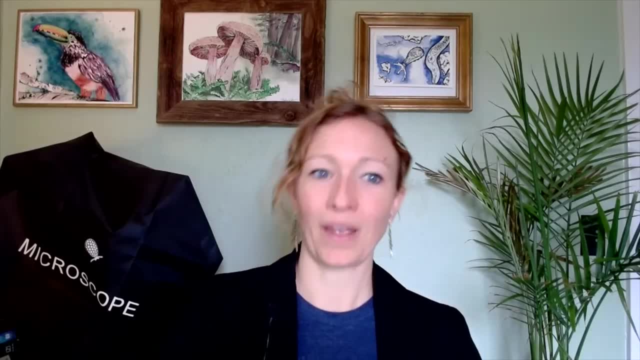 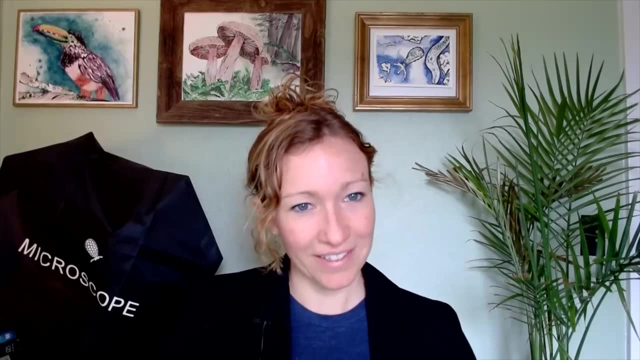 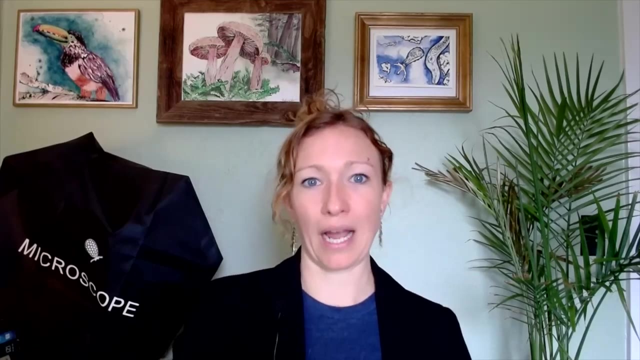 food web in those plant insect interactions, Dr Adam Cobb, a mycorrhizal agroecologist and soil food web science communicator. We will then have a live panel that we're calling our myco mind mill- Myco as in mycology. so all things fungal. 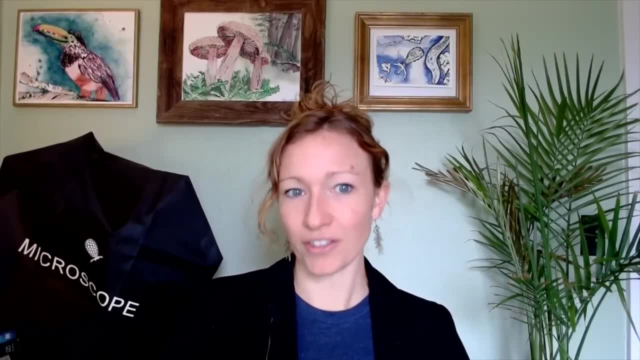 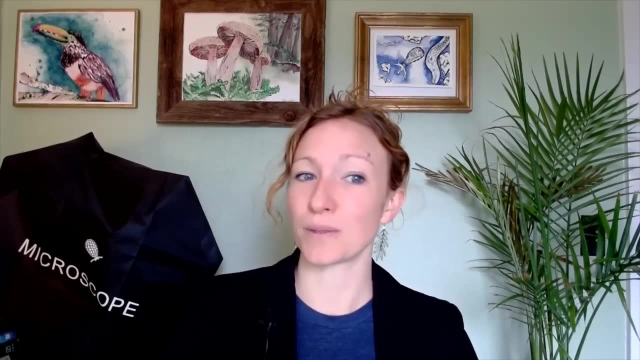 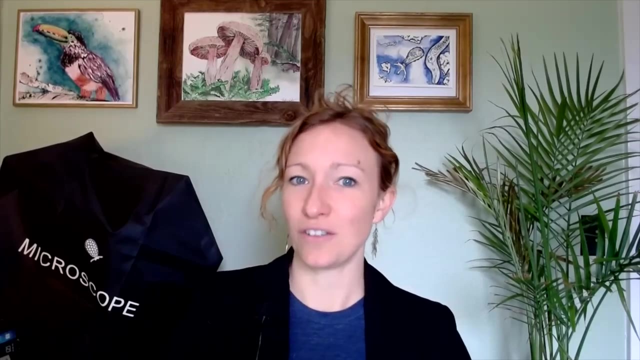 That will also include Merlin Sheldrake, the author of Entangled Life, and Peter McCoy, author of Radical Mycology and founder of Mycologos, Followed by even more talks from Dr Ted Turlings, chemical ecologist, professor at the University of Neuchatel, Also coming from 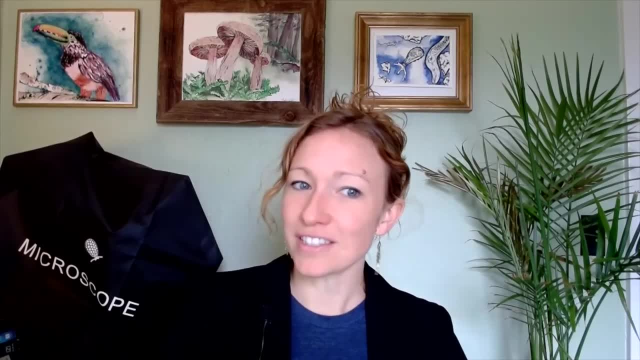 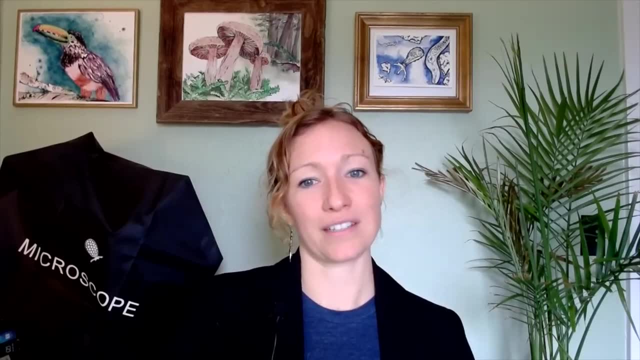 Neuchatel, we have Dr Edward Mitchell, a protistologist. Then we have Graham Lancaster, the managing director and founder of Southern Cross University's Environmental Analysis Lab, Then Dede Pursehouse, author, educator and founder of the Land and Leadership Initiative. 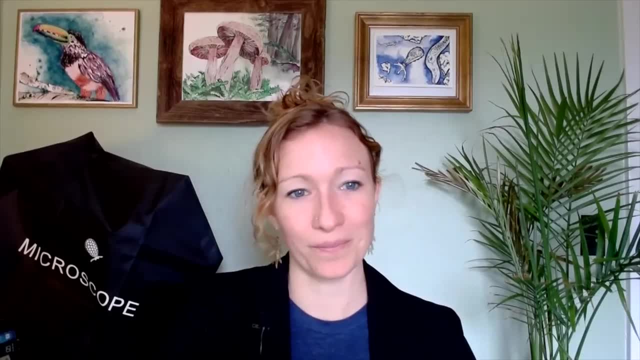 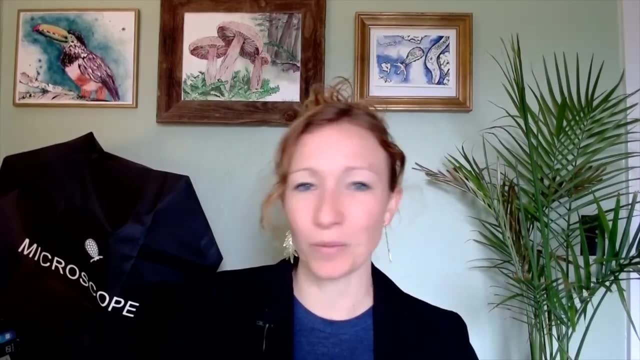 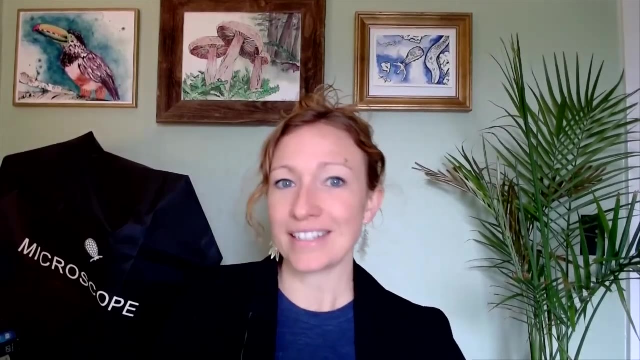 You'll get to hear more about the soil sponge from her, But first it is once again my honor to introduce Dr Elaine Ingham, an incredible woman and scientist and human. Her reach is far and wide and she never ceases to inspire. But since you've heard from 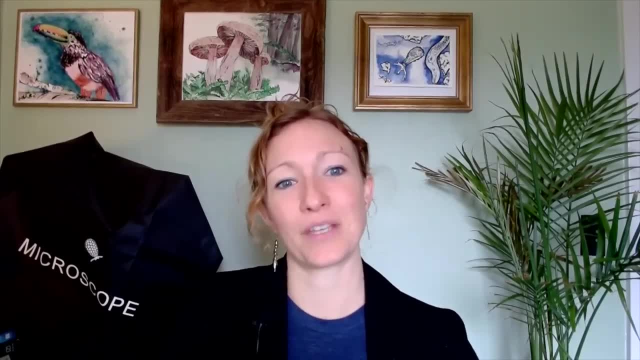 me about her several times, I thought I would share the mic. Here are a few staff who responded to the prompt. how has Elaine rocked your world in the field of regenerative agriculture? Take it away, staff. A student of the soil. 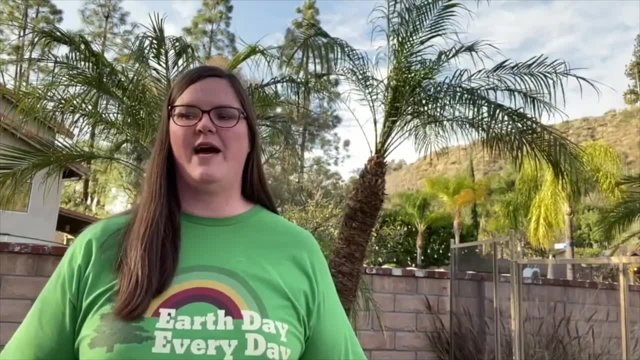 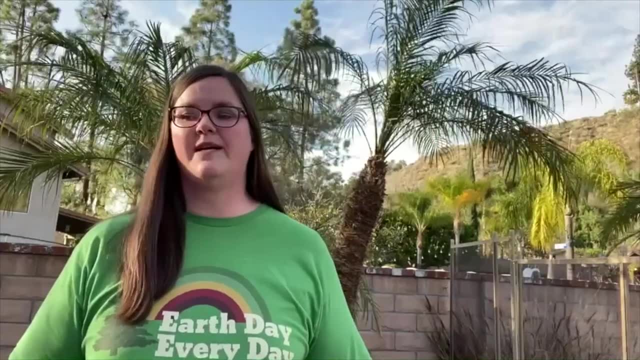 food web school once asked me how it felt to be working for a bad-ass female scientist. I told him it was the best feeling to be able to be employed by someone whose life work was making such a positive impact on our planet. I remember telling Dr Elaine that this student 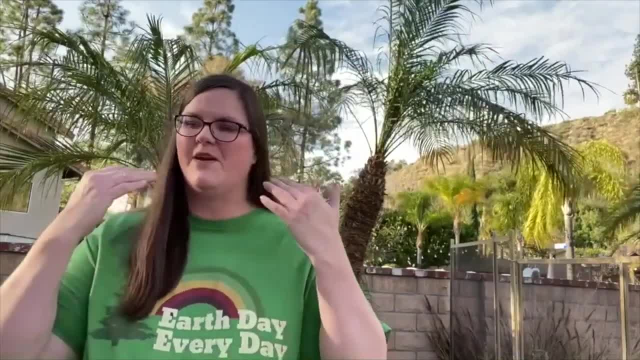 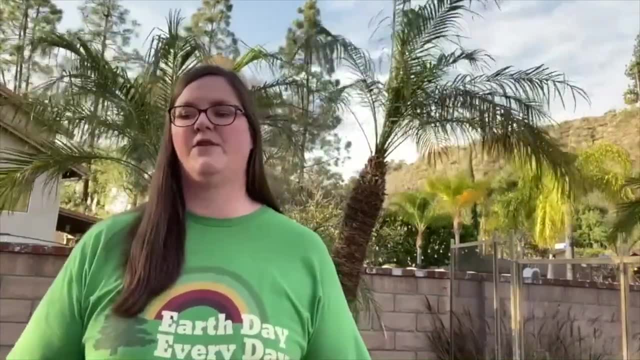 referred to her as such and I watched a smile slowly spread across her face as she said: that's right, I am a bad-ass female scientist. I can only hope she carries such pride with her always, because she truly is a change maker and someone future generations of scientists will love. 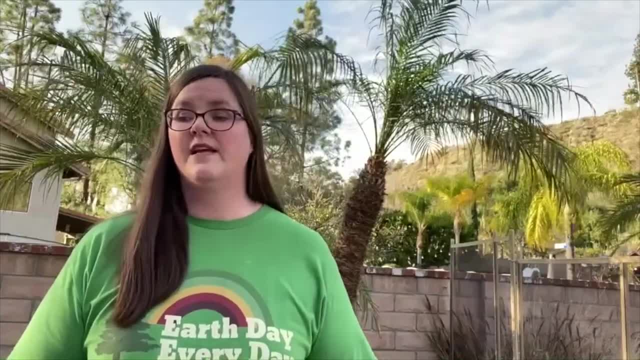 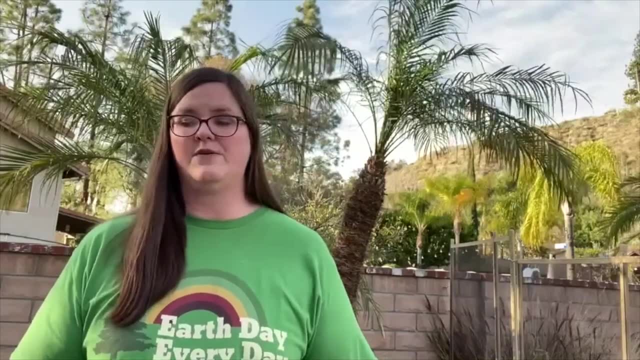 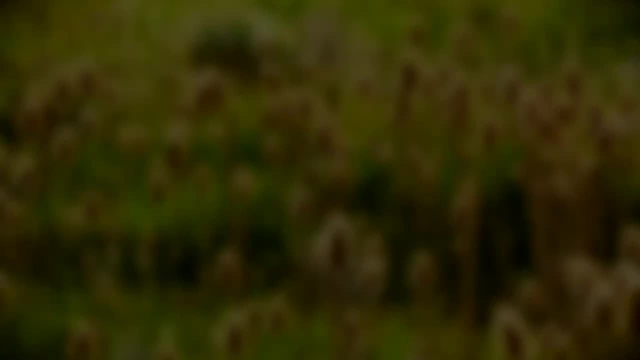 I'm so grateful. Dr Elaine created the soil food web school so that people around the world can learn how to restore their soils. I'm grateful that she is taking along the faculty and staff of the school with her on this amazing adventure. Dr Elaine is an inspiration for us in so many 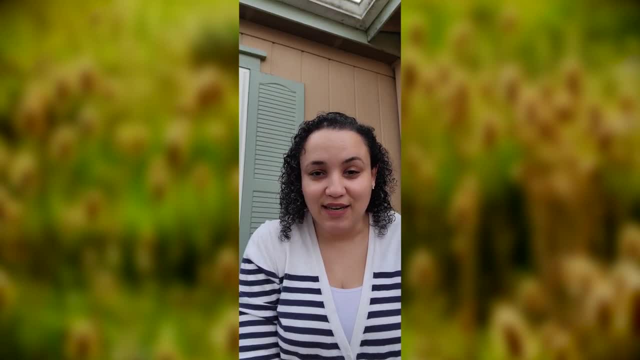 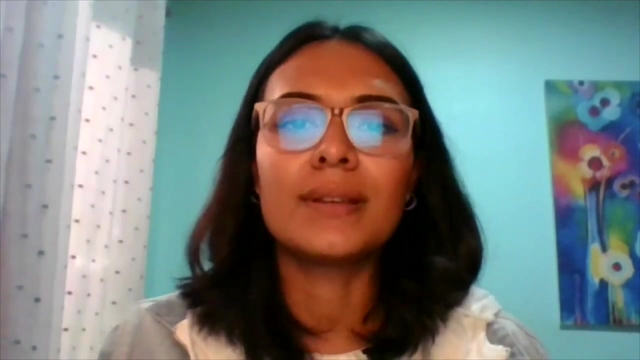 levels, but definitely my top three are her resilience, dedication and passion. Dr Elaine, thank you for showing us that. Please thank you. Thank you, Dr Elaine. Thank you for showing us that this is the way. Hello, my name is Marielle and what I find most inspiring about Dr Elaine? 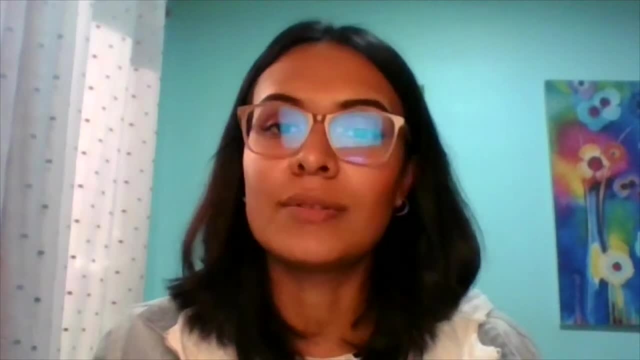 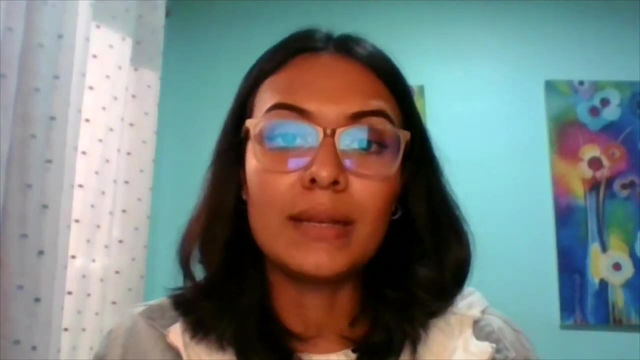 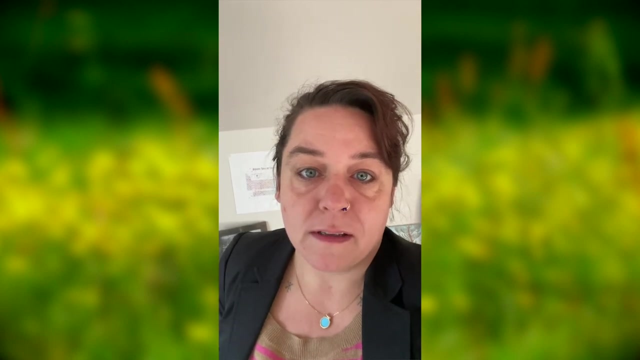 is her passion to communicate everything that she knows about the soil food web. She has allowed and created this great community for the people that really need that information, So that's what I like the most about her. Elaine's work helped transform and really even provide language around. 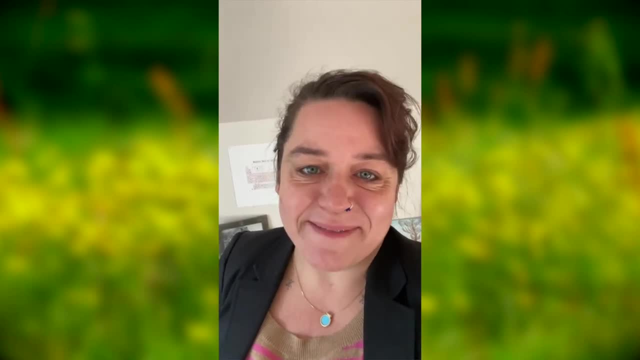 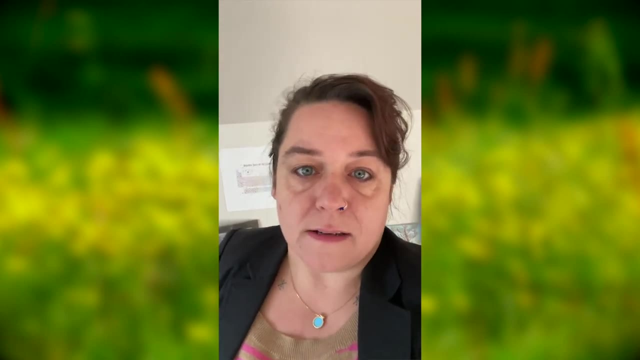 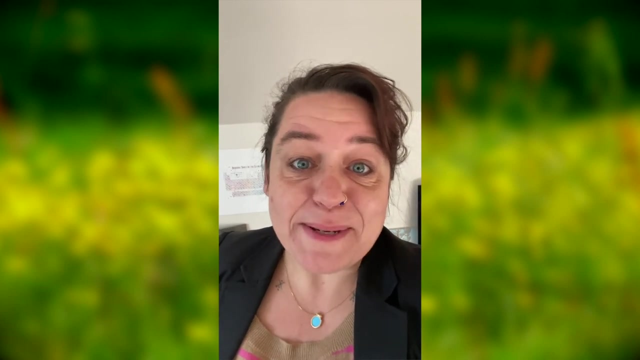 what I was repeatedly, recurringly observing in the field, And so I'm just so grateful for all of the tools and systems and understanding. Just even the stages of succession are brilliant. So I'm so grateful to be here and serve Elaine and the school and the mission to 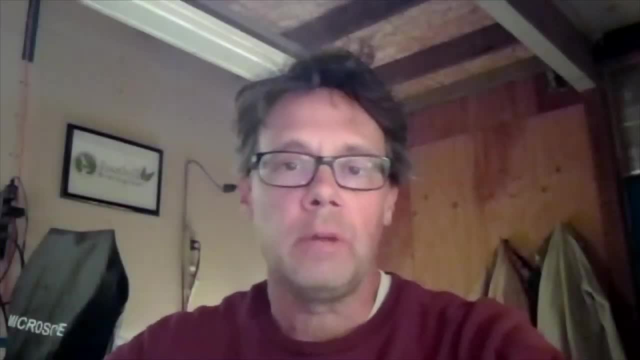 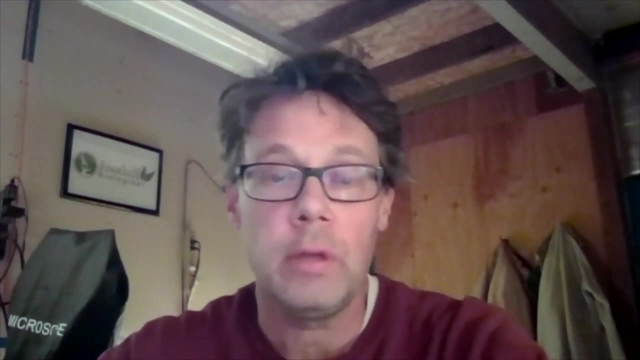 restore the world soils. To say that Dr Elaine has impacted my life, I think, is a huge understatement. The work that Dr Elaine has done is pretty much fills my life. This is what I do, It's my business, It's what I do here at the school and it's just amazing work. So, Dr Elaine, 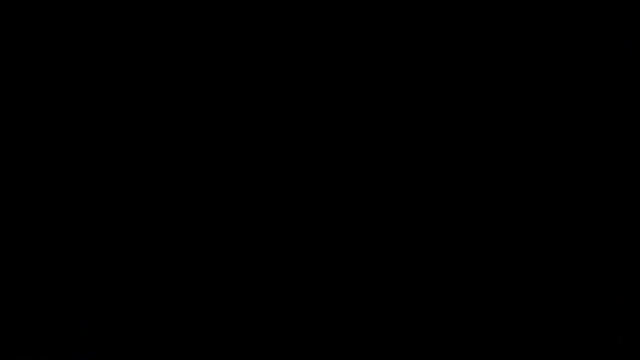 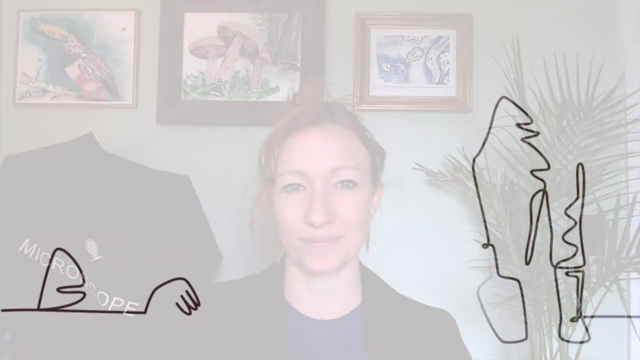 thank you, Thank you so much. Thank you for everything you do. And here she is, Dr Elaine Ingham, to share with us the science of returning life to soil. Dr Elaine Ingham, Director of theacon's office. 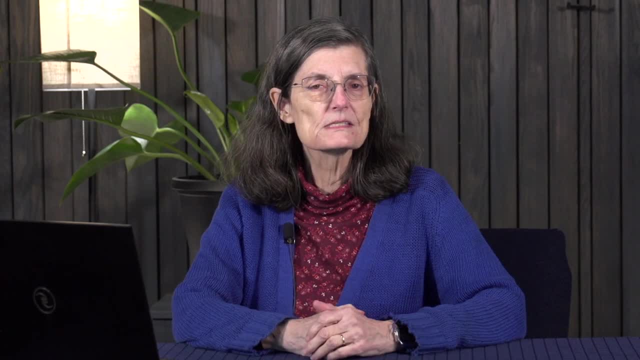 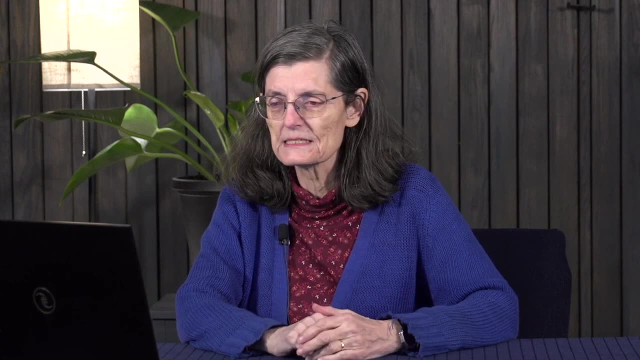 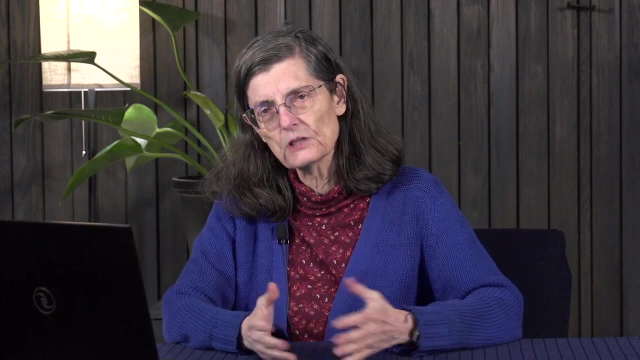 So welcome everyone to the third day of the Soil Summit. I've had about 30 minutes on each of the first two days of the Soil Summit. Today you get me for a little bit longer, Going to go over a number of things about the soil food web and talk about. 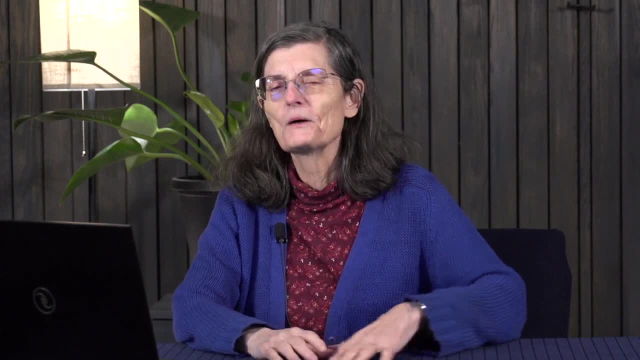 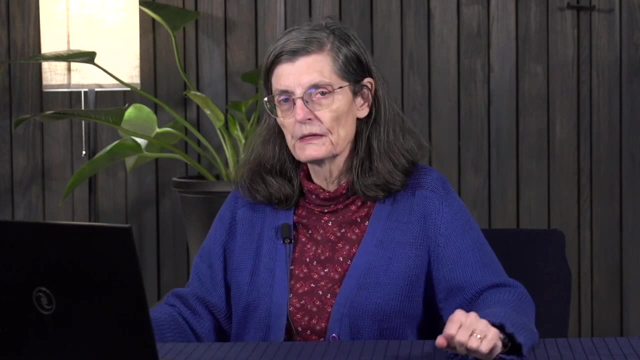 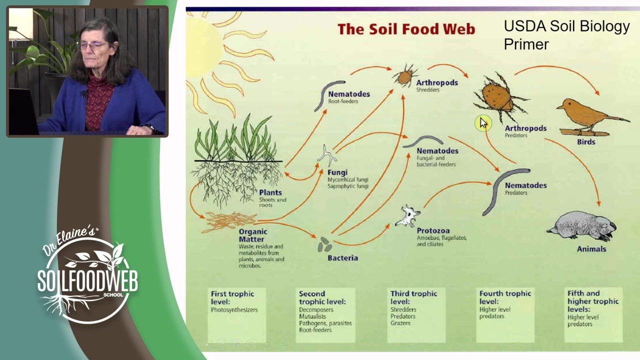 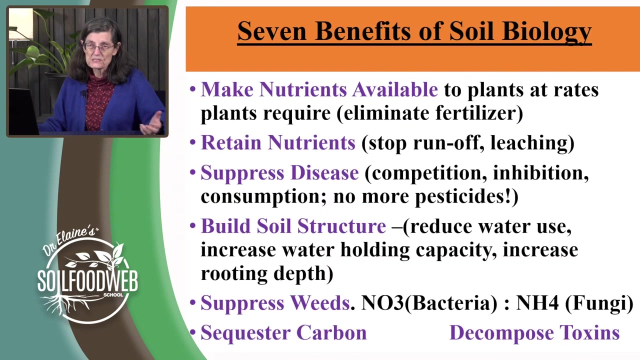 say, succession, talk about some case studies as well, so you can see the kind of things that we teach people in the school. so, looking at the food web of all the organisms, we've talked about many of these organisms, what they do, why they're important. so, moving on to the seven benefits from soil biology, we talked 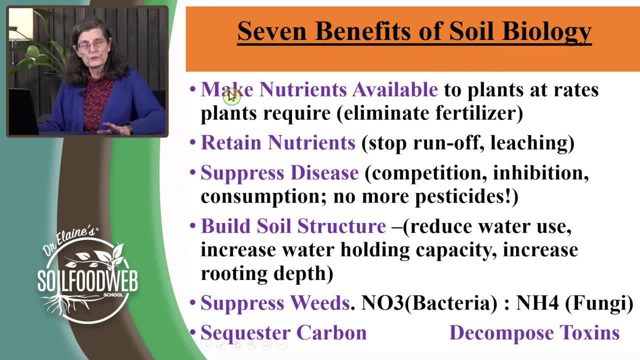 about this a little bit on the first day, where now, hopefully, you understand that it is this biology that make nutrients available, that convert plant not available nutrients into plant available nutrients. if you're having troubles with fertility in your agricultural field, you can pretty well bet that you don't have the biology in the soil, so you need to get that fixed. 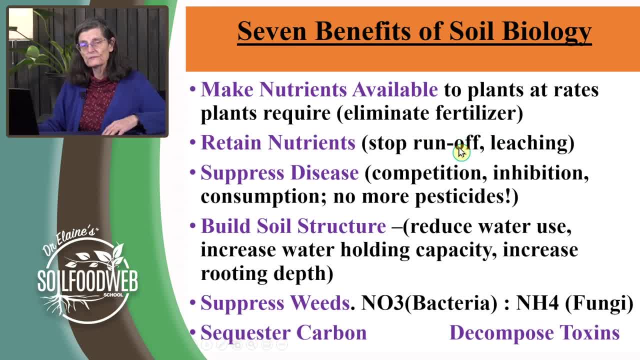 if you have a little bit of a problem with the soil, you need to get that fixed. if you have a little bit of a problem with the soil, you need to get that fixed. if you have leaching or runoff, if you've got erosion problems again, it's because you. 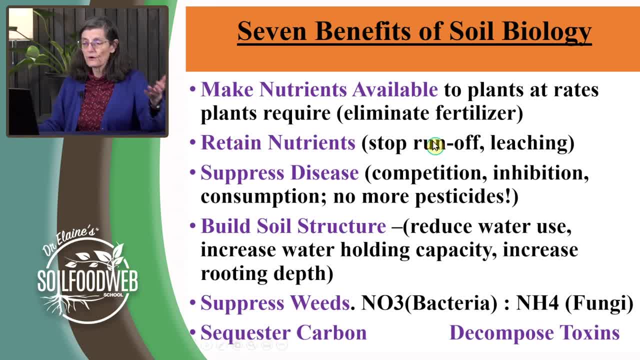 don't have the proper biology in the soil, and that means your soil itself is going to be lost from your system and most of the nutrients that you added as that inorganic fertilizer are going to be leaching instead of staying in place. you're going to be causing problems all the way through the watershed. these 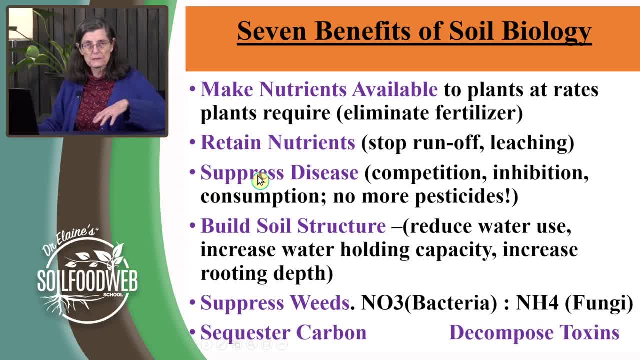 organisms suppress disease. they suppress the pests attacking your plants through the processes of competition inhibition and consumption. so you don't need pesticides and you don't need inorganic fertilizers. you don't need any of these toxic chemicals on your plants. so getting soil structure built, that's a major, important part of a. 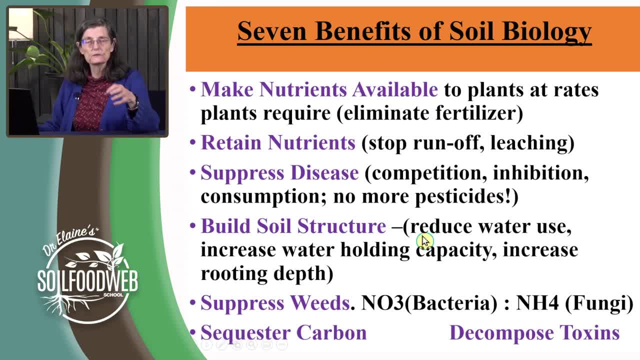 the work that we do with the biology is to build soil structure so you hold water against the flow of gravity and keep water in your soil. we increase the rooting depth, we get rid of compaction so that everything can grow deeper and deeper down into the soil, suppressing 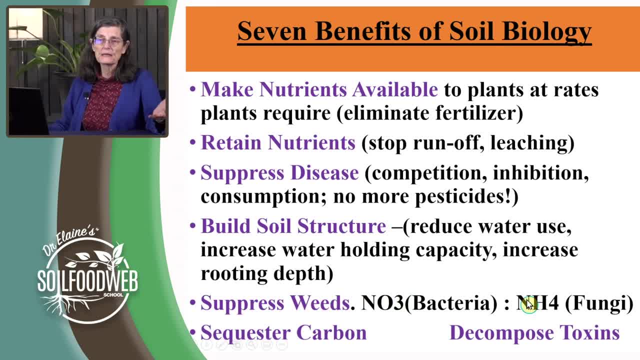 weeds, getting rid of the nitrate and making certain that your soluble nitrogen is present is ammonium instead of nitrogen, and that's what we're going to be doing with the soil instead of nitrate. you suppress weeds by doing that: sequestering carbon, keeping the carbon. 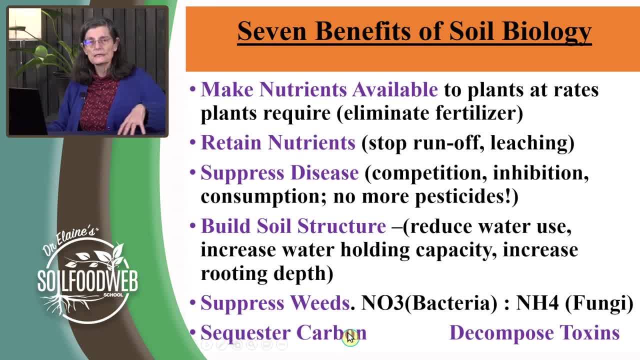 in the biomass of the microorganisms, in the organic matter that they release and maintain, carbon for hundreds of years stored in the soil, and then, of course, decomposing toxins. many of these microorganisms will decompose the chemical, um synthetic materials that we have put into the soil, and that's the only way to deal with them. 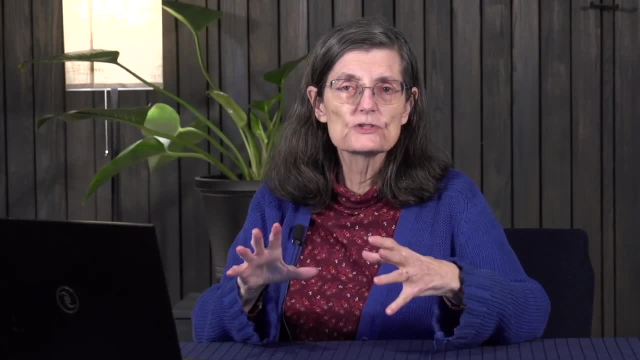 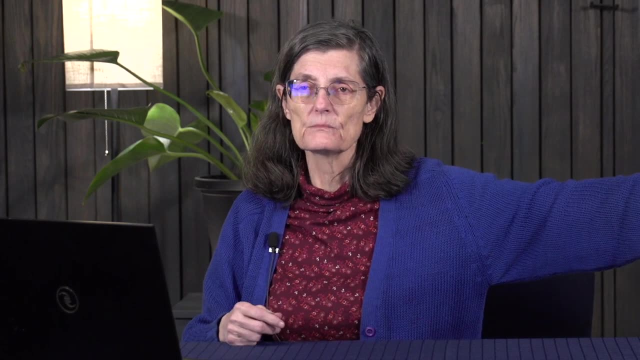 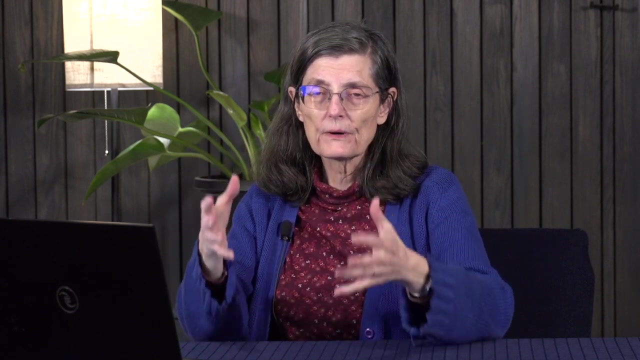 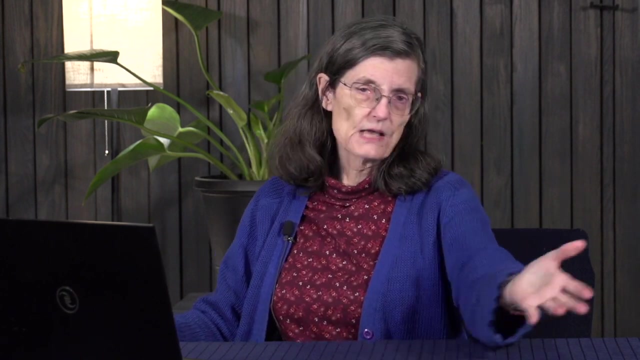 digging up all the contaminated soil and putting them into 55 gallon drums and carting those drums off and leaving them someplace just means we've got two contaminated sites instead of just one. deal with the problem on site and there are ways of dealing with that. uh, and i'm- some of the speakers have spoken about that. i'm. 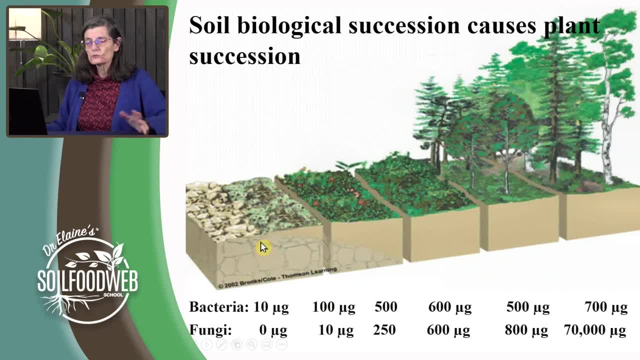 sure we need to understand what drives the system from this very nothing, hardly going on, no food being produced, no plants growing. how is it that you move from bare soil to ever more productive systems as you go through time? what causes this change? and it's a bit of a bootstrapping system. 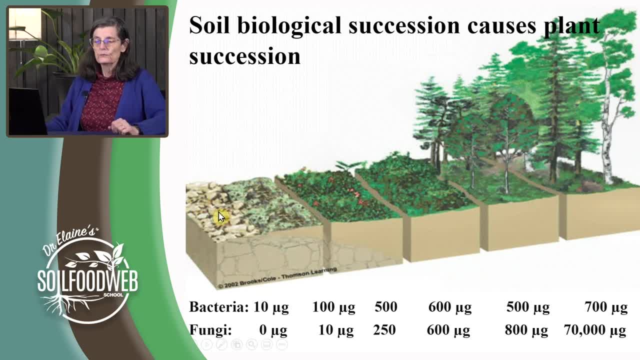 that's going on here, where you have no organisms growing in that soil after catastrophic, catastrophic disturbance, for example, like a forest fire that causes the soil temperature to increase to 600 degrees fahrenheit, or you have a mudslide and anaerobic materials are left on the surface of the soil all the way. 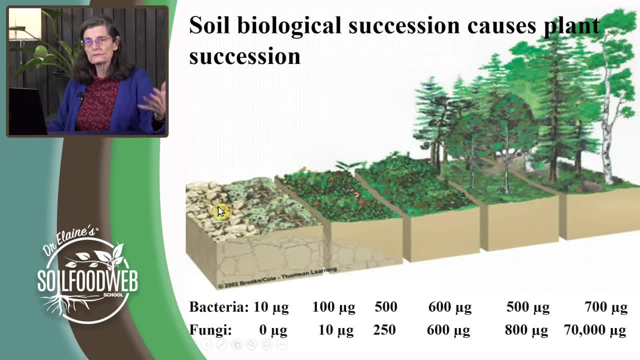 along that mudslide, all of these horrible, catastrophic things that can happen when we first start off, typically only photosynthetic bacteria growing in that bare soil. nothing else can grow because there are no organisms to cycle nutrients and start this process along until we can get some of the photosynthetic bacteria. 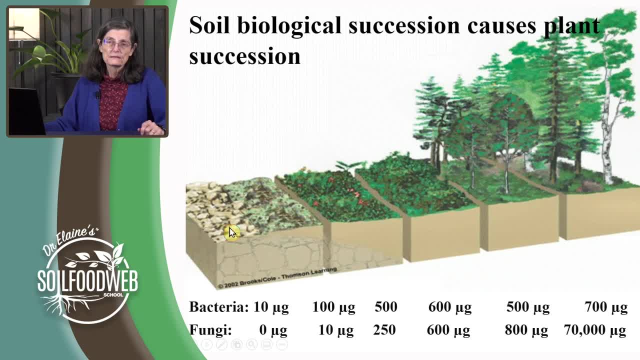 come back and as the photosynthetic organisms add their biomass to that soil, you'll notice that here, where we're tracking the bacteria and the fungi, we've got 10 micrograms per gram of soil of bacteria, but absolutely no fungi at all, because there are no foods yet. 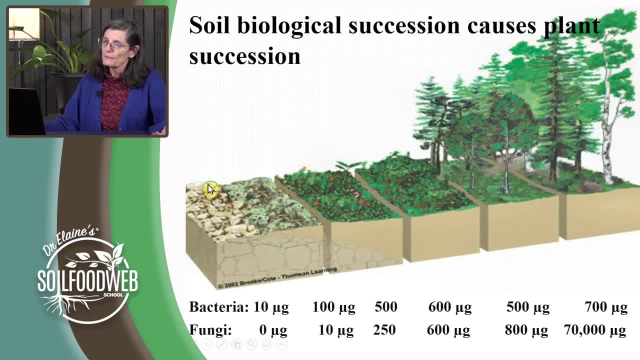 in the soil. so we don't know how many of those organisms to grow. so bacteria, photosynthetic bacteria- are the first organisms that come into an area that has had a catastrophic disturbance. as those photosynthetic bacteria grow, they're producing lots of food resources for our fungi. 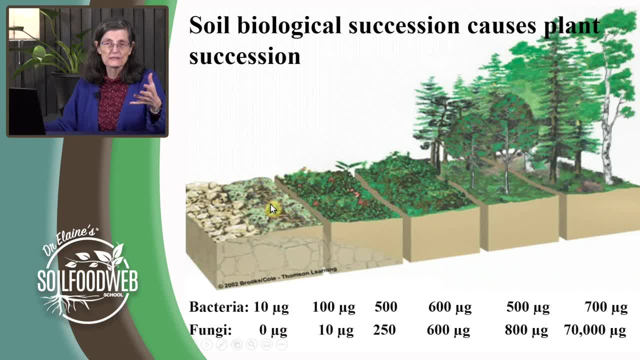 and so eventually, as a photosynthetic mosses, the algae organisms come in and start to leave behind biomass. now you've got some foods that the fungi, the very early succession of fungi, can grow on. so you'll have a fungal to bacterial biomass ratio upwards of 100 micrograms of bacteria to maybe five or ten micrograms of fungi, very bacterial dominated. 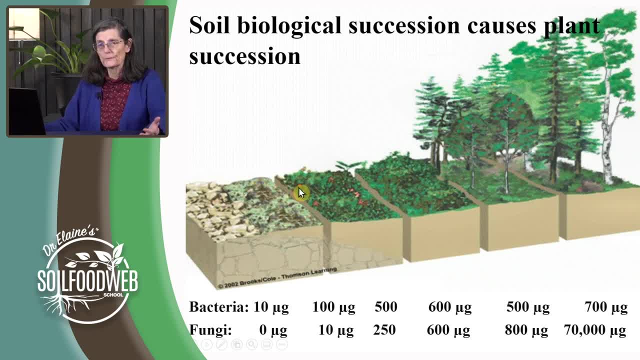 and so these are a perfect place for weeds to grow, improve the pH, are a whole series of organisms healing ouritzoc 압 and because it's strictly bacterial- aerobic bacteria- it means nitrate is going to be formed, and so you'll find a lot of. 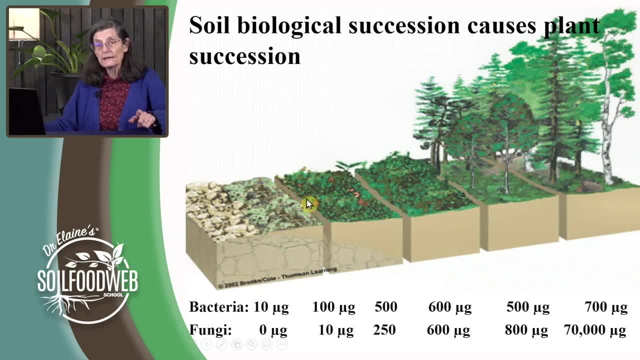 the weedy species at this stage of succession. but because you start to have some weeds growing in this part of the successional process, that means cellulose is being produced, and pretty much only cellulose when you're dealing with these early successional plant species. but it's enough to start changing the 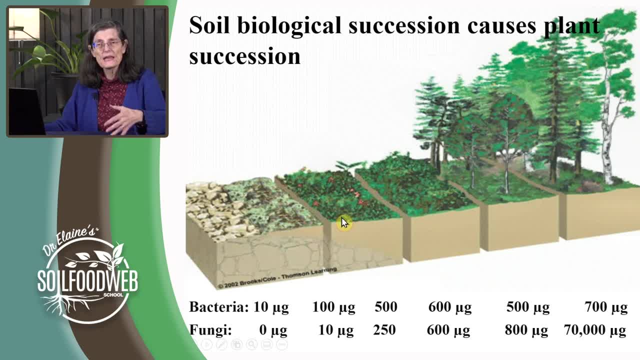 biology in the soil, which will then change the set of plants that can grow here. so now we have early successional grass species, we have the coal and the kale crops, the different kinds of brassicas, for example, growing in this early successional system. riparian plants usually are at this stage of. 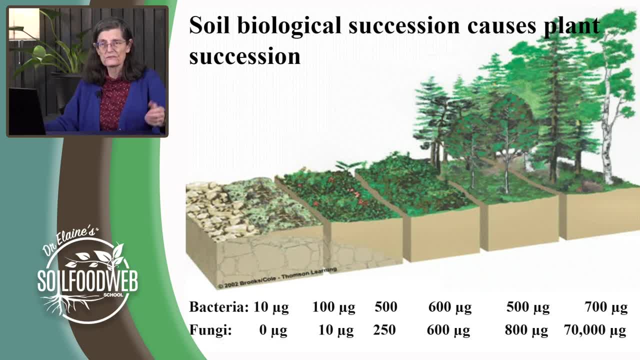 succession, as are the wetland plants, but in terrestrial systems. we're going to continue to increase the amounts and types of cellulose that are being produced. some lignans start being produced, and so you're going to move along in the process of succession. notice now that you're at five hundred. 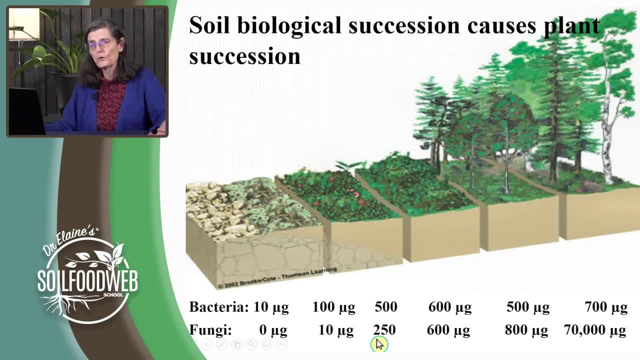 micrograms of bacteria and 250 micrograms of fungi. So fewer weeds are going to be growing in this system. There's still a few, but you've definitely suppressed that particular problem. Well, because there's a lot more of these fungal foods being made. that means fungal biomass will. 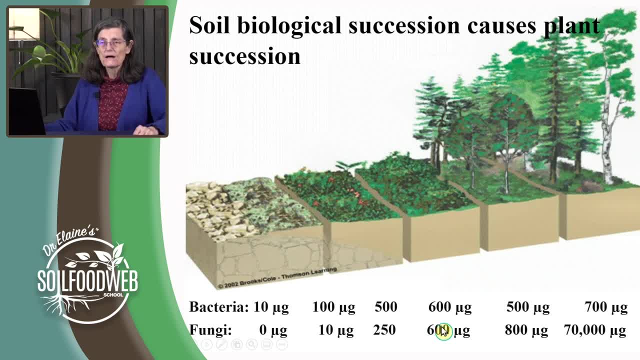 increase. So 600 micrograms of fungal biomass to 600 micrograms of bacterial biomass. And the typical kinds of plants that are going to be growing at these ratios are going to be our highly productive grasses, the row crops that we grow, so corn, barley, wheat. 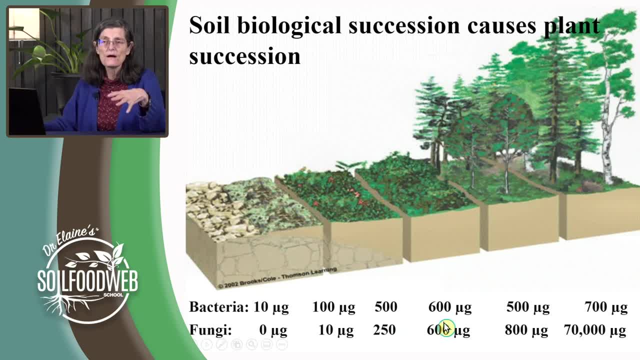 oats. they are all one-to-one ratio of fungi to bacteria. The potatoes they're in this stage, so they have still bacterial dominated, but you're getting much closer to like a 0.6 to 0.8, so 0.6 units of fungal biomass to every one unit of bacterial. 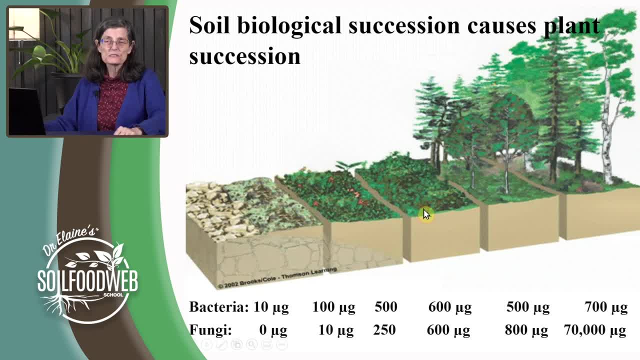 biomass. So one of the interesting things that we find is that as long as you keep these two balanced like this, you can. You can get higher and higher and higher numbers of bacteria and fungi and as long as they remain balanced, you're going to continue to grow higher and higher amounts of corn barley wheat. 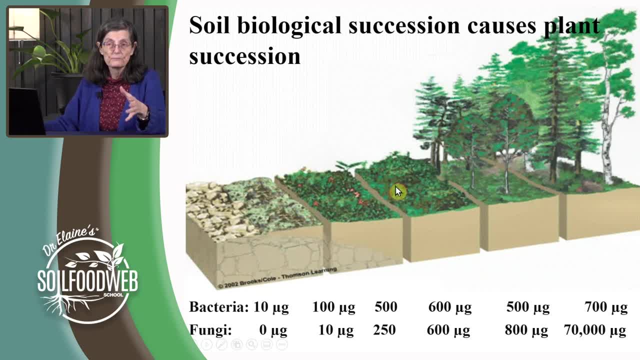 those kinds of mid-successional row crops. Some of the most productive grasses grow at this stage and many of our herbs, our different kinds of spices, also grow at this stage of succession. Now, as these guys are growing very well, growing even more fungi, you'll start to convert from this. 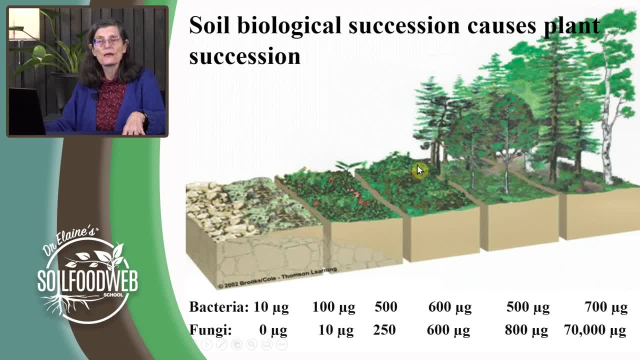 mid-successional stage into shrubs and vines starting to grow. So on the fungal dominated side and now things like grapevines, blueberries, blackberries, strawberries. that's the right place for them to be able to grow With time, because you've got more and more woody types of materials being made by the plants here. 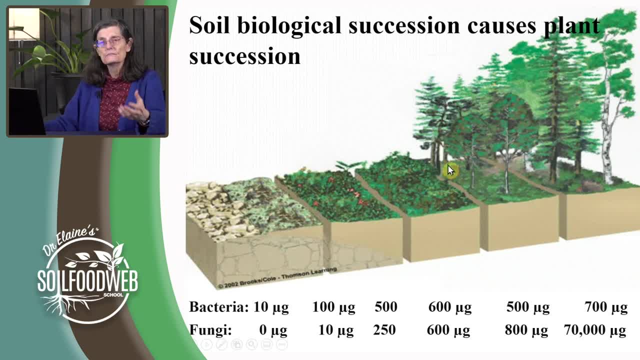 the microorganisms will respond by developing ability to decompose these more and more complex food resources in the deciduous trees. So that's what comes next. As time goes by, you go through that succession from early successional deciduous trees to later successional deciduous trees. 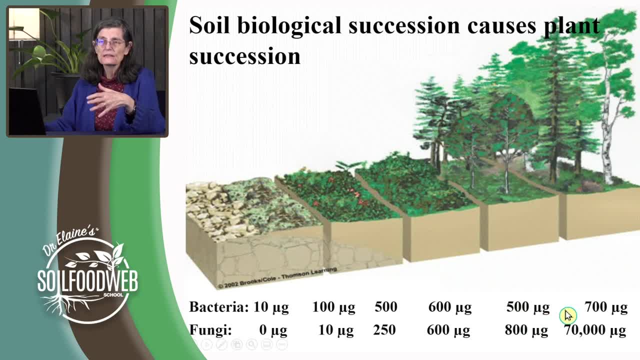 And then, finally, you're going to go over the edge into conifers. Old growth forests are on their way, as long as you don't disturb. So, as you're going through succession and you see things happen in this way, can you increase the speed at which these converges? 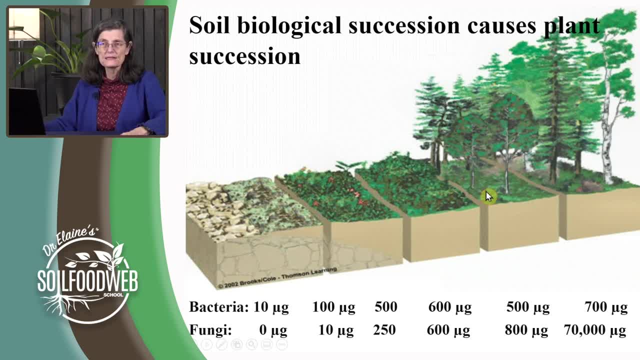 Can you make these conversions to the next kind of plant, the next kind of productivity occur? And the answer is yes. We can start out here, put the proper biology into the soil so we can immediately start growing potatoes Or immediately grapevines. 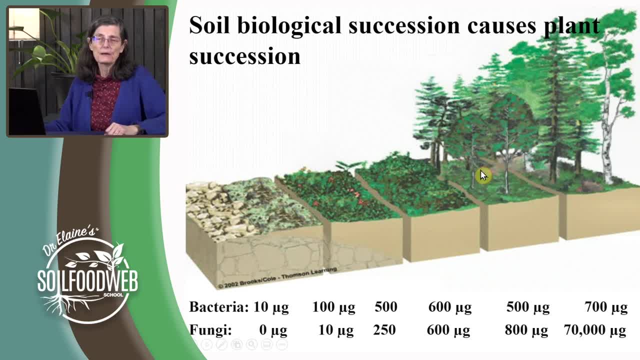 Or even, if we wanted to, if we could get enough of the biology into the soil, we can start growing trees almost right away. So we can do this kind of jumpstart of what's happening in systems where we don't want to have to wait. 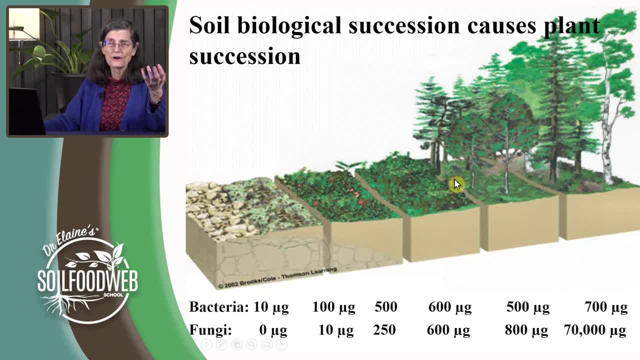 35 or 50 or 100 years to get into a productive vegetable system. When we're looking at these old growth forests, you'll notice that the bacteria are really pretty much still in the same range. It's only 700 micrograms of bacterial biomass. 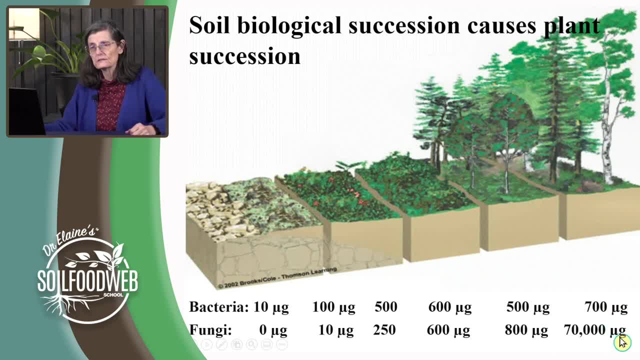 But look at the fungi: 70,000 micrograms. If you're a little bit lower, this could be 7,000 to 7. So that ratio of fungi to bacteria can tell us about what's going on in the soil. 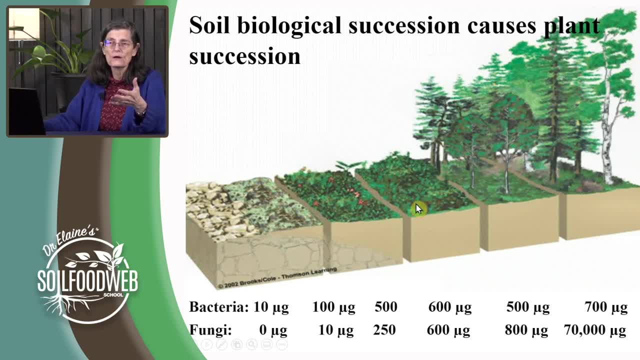 What plants should you be able to grow? And if you want to grow, if you want to grow kale, you better not have a soil that has 500 micrograms and 800 micrograms of fungi. You're going to need to come back into this range of fungi to bacteria. 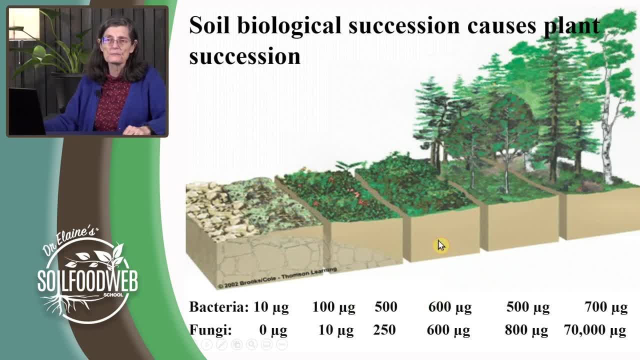 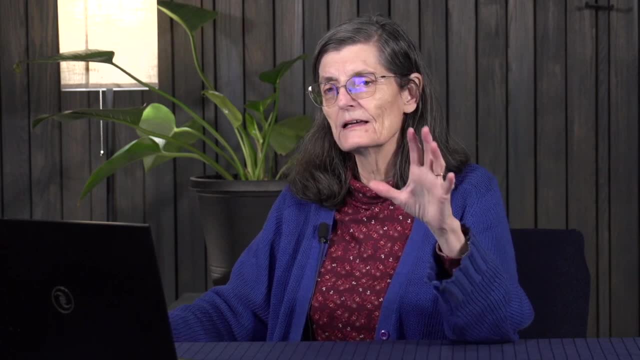 Well, what if you're here growing some good row crops and somebody wants to come in and grow grapes? Fine, just more fungal food is all you have to put in. So understand that, Understand that. Understand the needs of your plant as well as what's present in that soil is one of the starting things that we have to do. 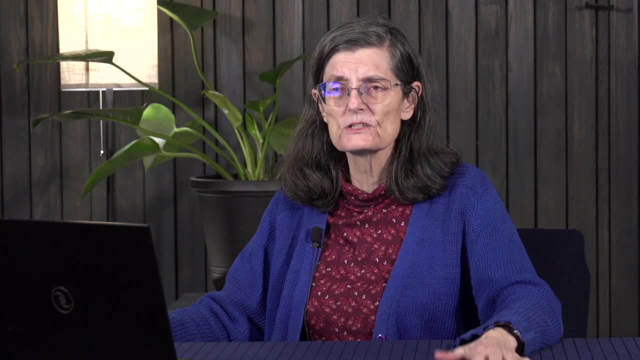 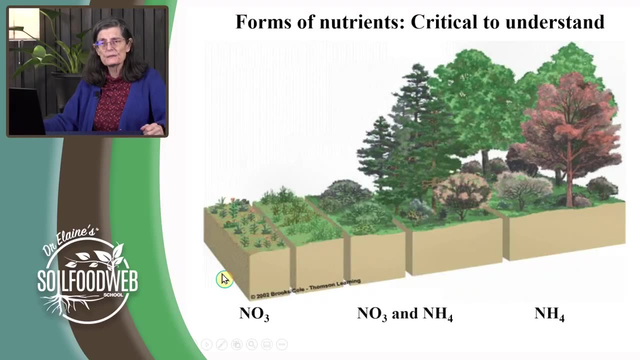 What do we have to fix in order to get this system jumpstart to what you want to grow? And then remember that as we go from a very bacterial-dominated system where the only kind of soluble nitrogen is going to be available is when we're totally bacterial-dominated. 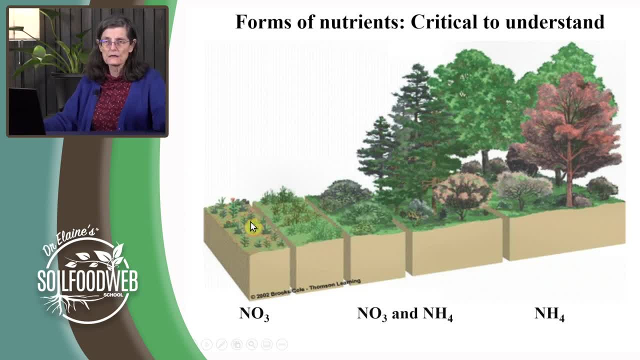 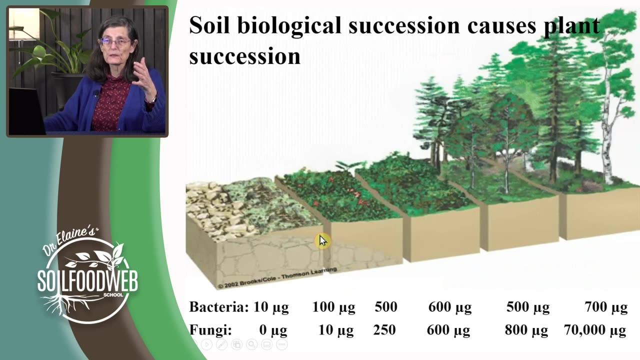 Weeds grow in these systems easily. You know most people think of these as weed fields. Well, how do you quickly get back to a more productive system? You've got to start getting the fungi back into the system. It's not a lot if we go back to this picture. 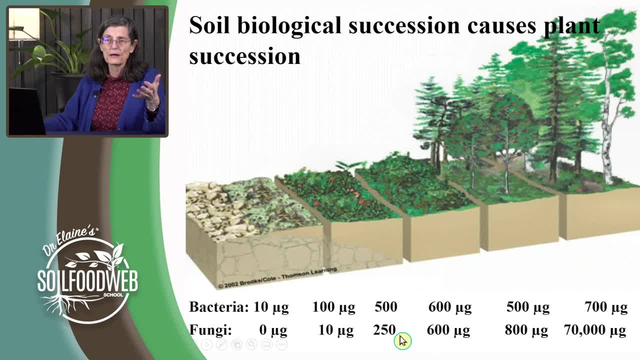 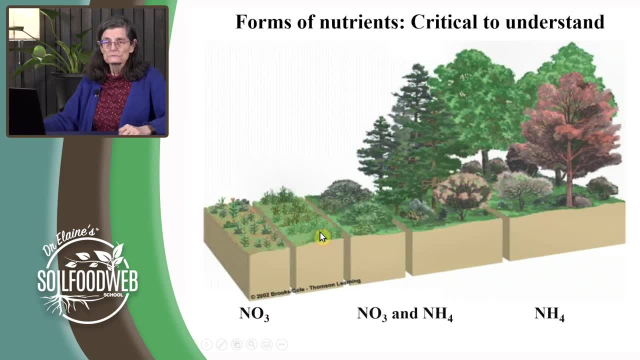 Now the fungal biomass is significantly less than the bacterial biomass. if you want to grow the army of fungi plants without weeds, keep going up more and more fungi. equal biomass of nitrate and ammonium are perfect for row crops. you wanted slightly more ammonium than. 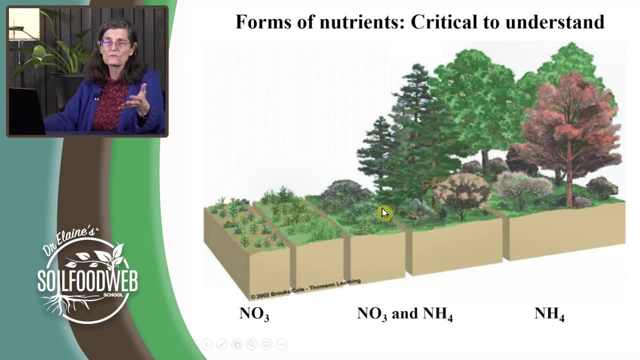 nitrate. if you're trying to grow vines and shrubs then it's got to get quite a bit more ammonium present in the soil. and when you get into old growth forests, there was a belief for a long time in the world of forestry that there was 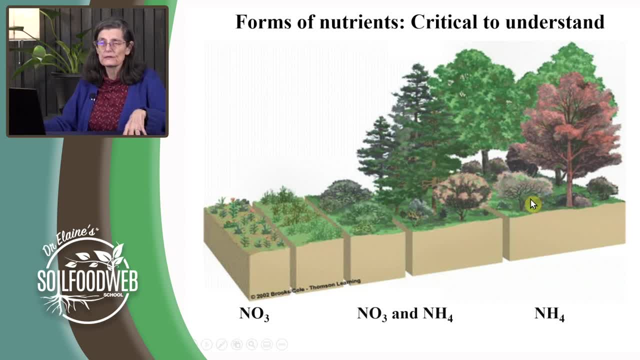 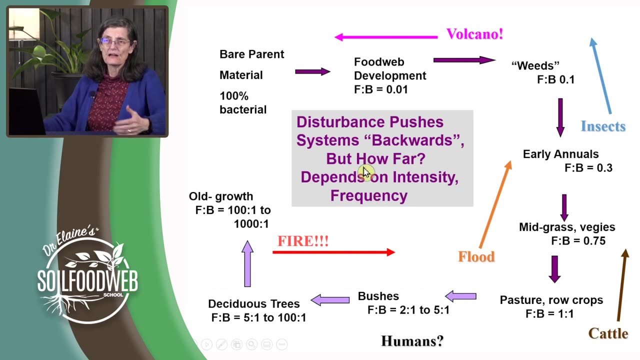 never any nitrate in those soils, when in fact it's just the conversion of all those nitrates into ammonium that helped these trees grow in a highly productive fashion. so another way of looking at all of this is: you know, this is the course of succession taking us around to 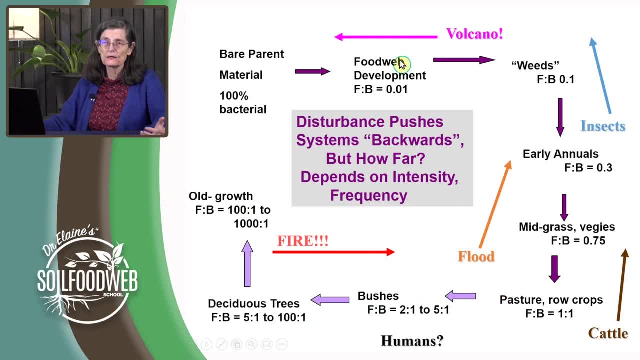 the old growth forest, all the steps that we just talked about to get yourself up to that old growth forest. well, how often does Mother Nature move this around? so you go 10 or 20 or 30 years in here, even more years to move through this stage of. 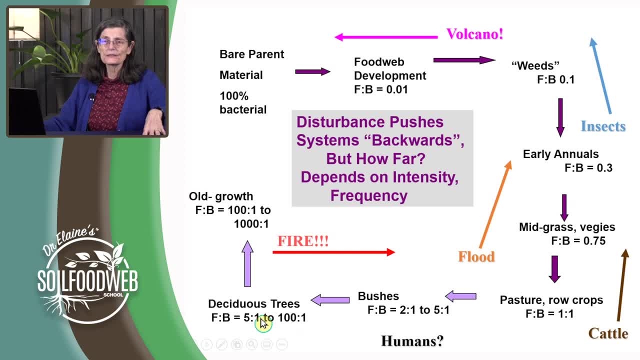 succession even more. you know: 100, 120, 200 years to start growing an old growth forest. how often does that happen? never, because usually what's going to happen is you. the course of succession is pushing you this way, and then some disturbance happens, like a massive amount of insect pests come through and 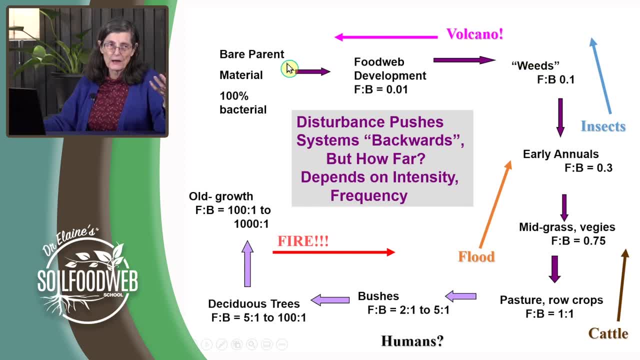 you go backwards and then a volcano happens and you go backwards and then you start going again and then you get up to here and a flood comes along. so you're going to go backwards. okay, the mother nature, nature starts building more and then a disturbance happens and yeah, they're finally old growth, forest and 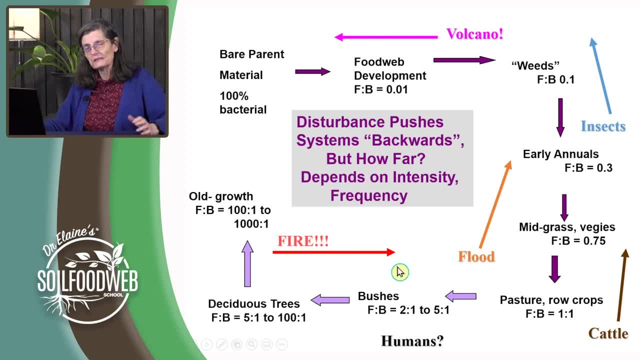 then a fire comes along. so this is well from Mother Nature's point of view. this is constant yin and yang, back and forth. how long did you leave something undisturbed so that succession can keep happening? well, could we come in here at a very early stage and add the organisms back in here, so that we can 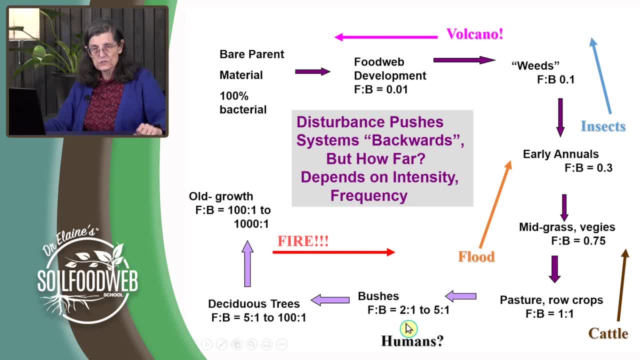 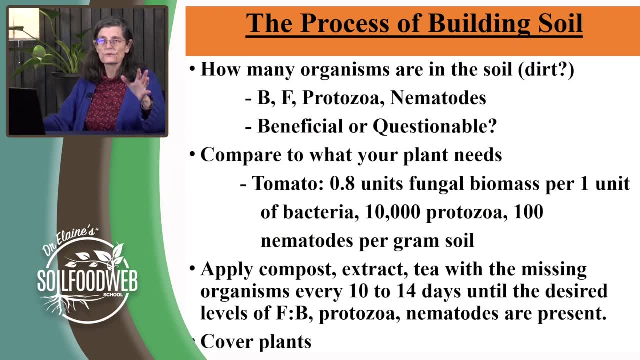 get the system that we want, and so far experiments are showing that that's true. so get the biology right for your plant. so here we are: the process of building soil. job number one is to figure out how many organisms are present in your uh dirt, or maybe you're lucky enough to have soil or part. you're part way along, so we've got to learn. 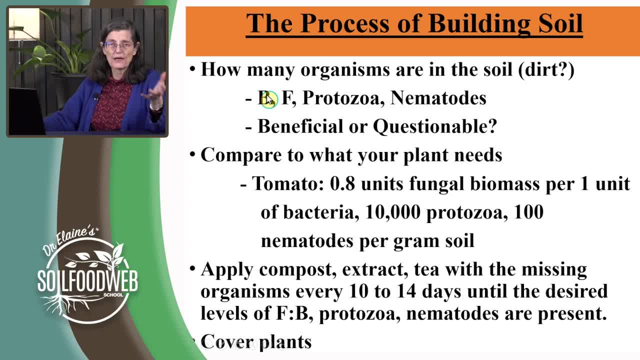 all about the bacterial biomass. what's present? do you have actinos? do you have rod shaped organisms? do you have the bad bacteria and not the not the good? are your fungi good guys? are they bad guys? do you have the mycorrhizal fungi, protozoa? do you have both the flagellates and the amoeba? 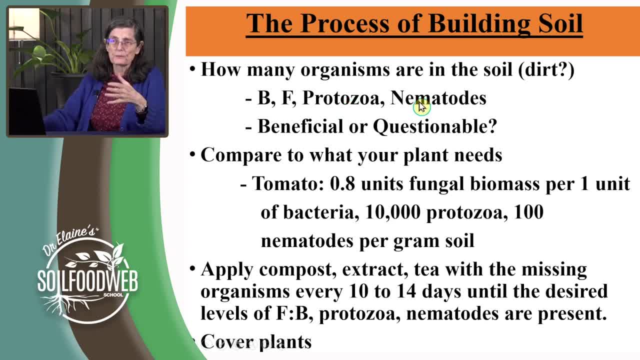 do you have the bacteria feeding nematodes, fungal feeding nematodes, predatory nematodes, the good guys, or do you have just root feeders? do you have the beneficials or do you have the questionable things that you did not want to see? that root feeding nematode, but it's there. 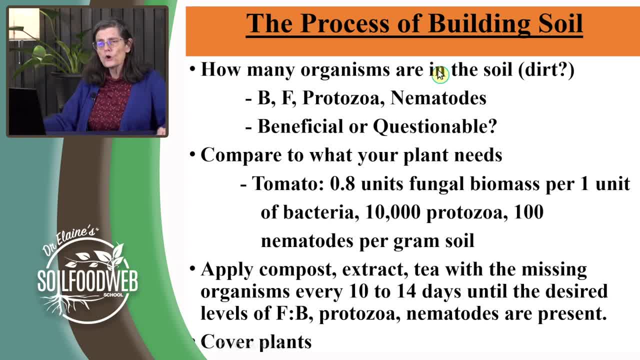 and you have to pay attention to it. so now, knowing what's there, now we're going to design a program that's going to get you to where you want to be as rapidly as possible. so let's say you want tomatoes. you know that you need 0.8 units of fungal biomass for every one unit. 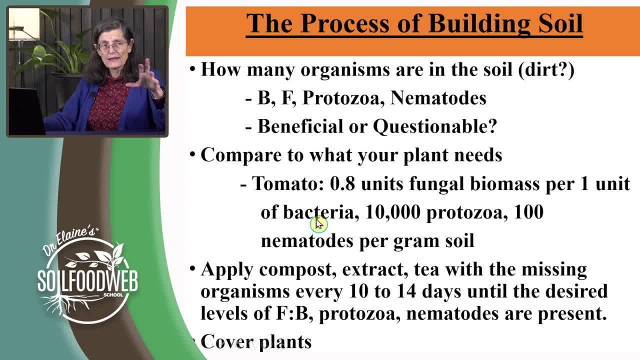 of bacteria, and so that's what you're aiming for. you may have to be putting in a huge amount of fungal material, an inoculum of the different kinds of fungi. you may have to put in some more bacterial foods as well, but exactly what you want for each of those plants that you need the most fungal of. 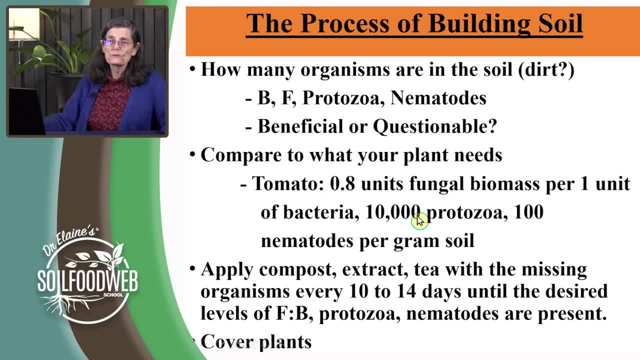 the different kinds of fungi. you may have to put in some more bacterial foods as well, but exactly what you need. so I'm going to show you how to determine when they start to grow in the you have to do to reach the goal. so we're going to apply compost, hopefully compost with lots of 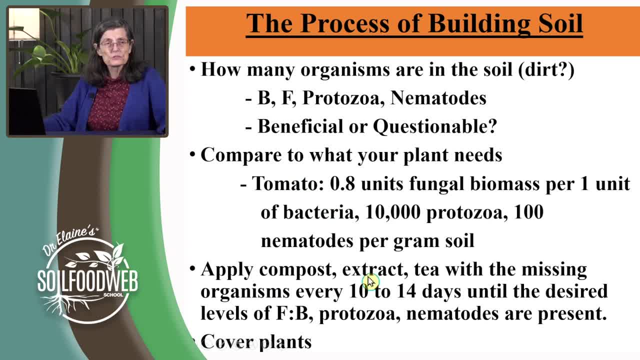 good fungi in there. we can use some extracts. during the growing season we'll go out there and apply liquid compost. all we do is extract the organisms out of that compost into the water and now we'll go out and apply them tea where we've grown these organisms, in the um, in the 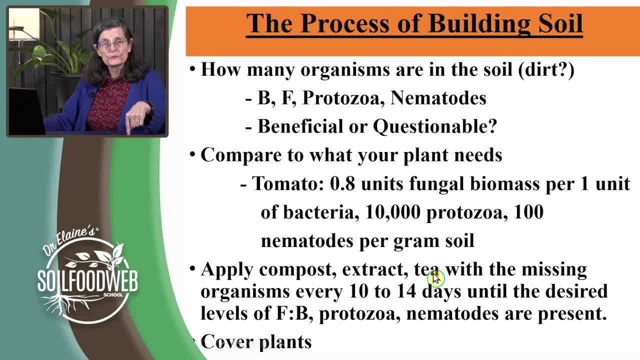 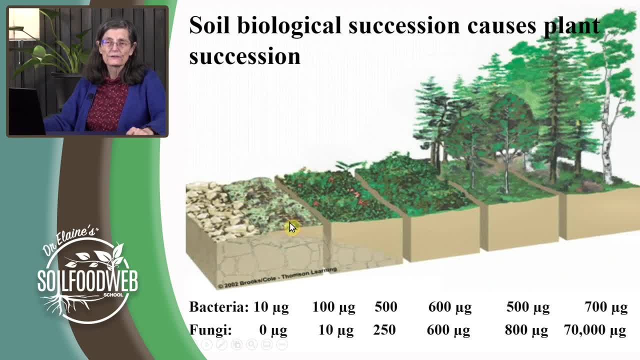 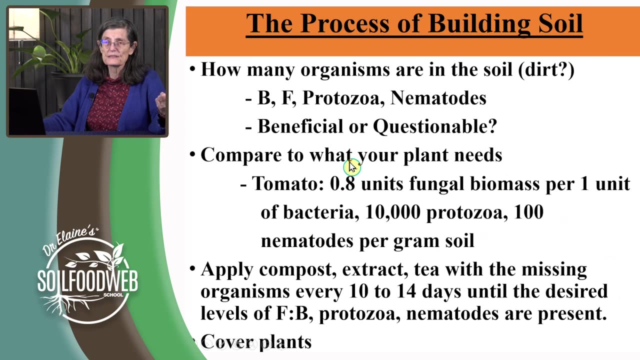 brewer by adding food. what kind of food are you going to put into this soil? if you are here, what are you going to put into this system to start growing tomatoes? both some bacteria, but mostly fungi? right, make sure you've got the protozoa. make sure you've got the nematodes. 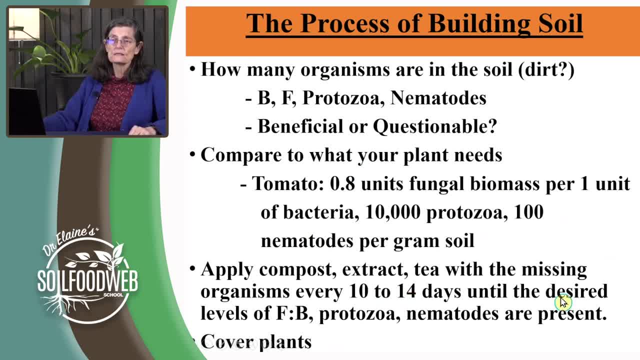 you want to be checking every 10 to 14 days until you get the soil to that desired level of fungi, to bacteria, protozoa and nematodes. we like to use cover plants now. ground cover might be a good term for us to be using instead of cover of crops. i don't like cover. 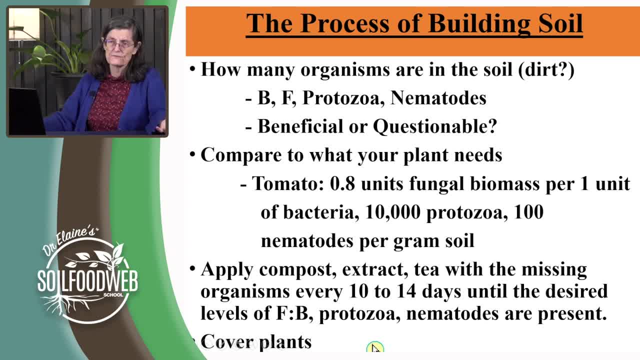 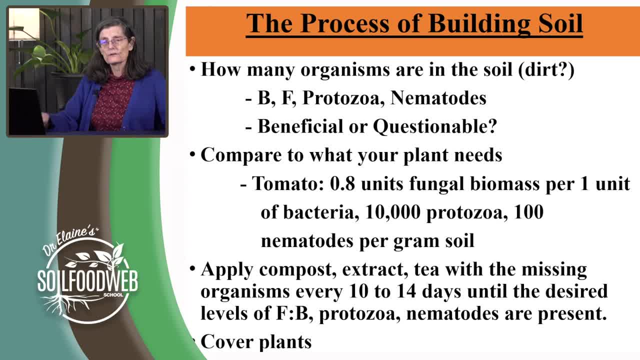 when it's landing and starting to melt, you're not going to have impacts on that soil to the extent where you, where you have only bare soil. we want to make sure in the springtime, that we've got these plants coming up just as early as you possibly can. they're perennial. they need to be there growing for those first. 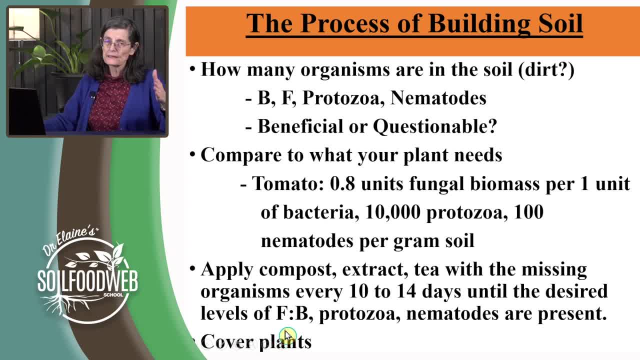 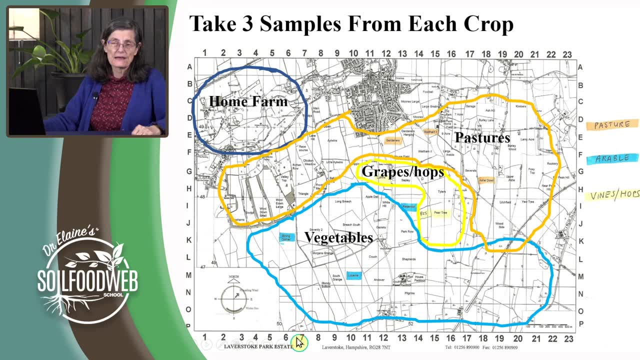 rains that you get in the springtime, and some of them can just bash your soil and compact it to really horrific levels. so you want to make sure that you've got cover plants that are going to protect that surface. so here's an example of a really large operation where this is their home farm, where they grow all their vegetables. 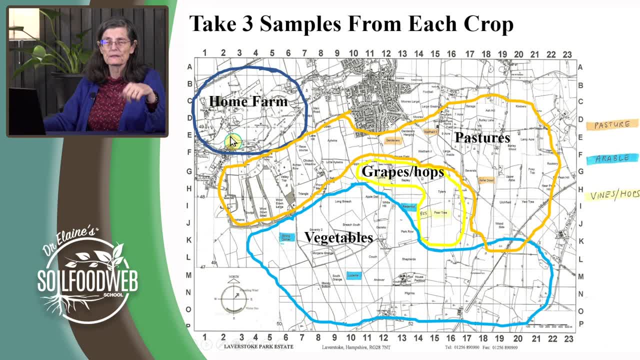 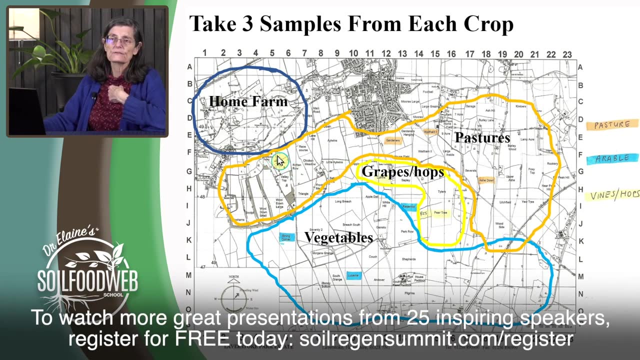 all of their foods- chickens and a few little pic率s and things like that in the home farm. but when we get out and we start looking at this scale of production, all of the hogs are down here, all of the sheep are here, all of of the you know. you know what all is in there and you want to start taking a look at what's. 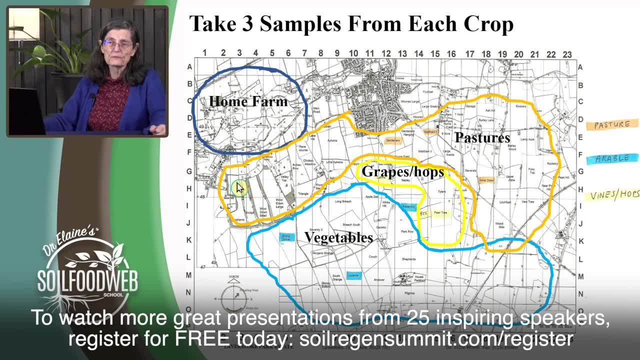 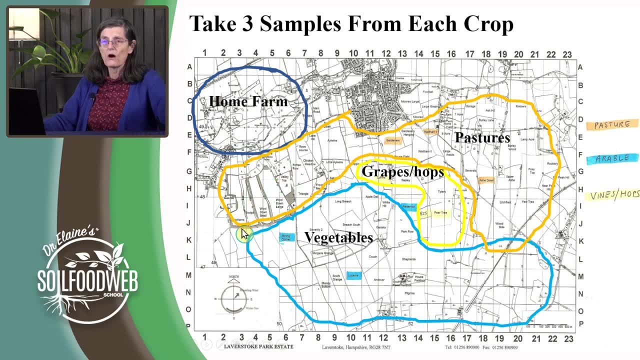 happening in all of these places. well, so you're going to take a sample from this paddock, a sample from here and a sample from there, so you're covering all of the area that the hogs are in, and do the same thing when you're looking at the next set. same thing when you're looking at where. 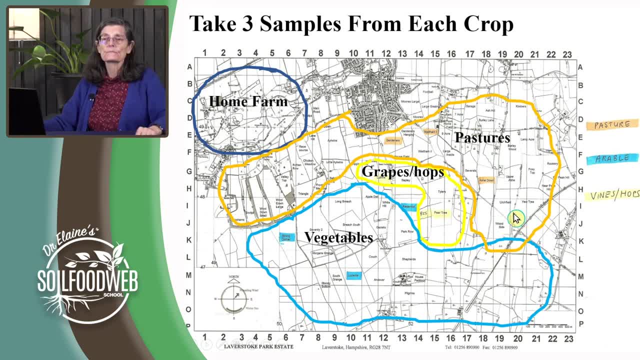 the horses are being kept or the llamas are being kept, where you've got grapes and hops growing. you want to mark that area- that's the grape vines- and you want to be taking at least three samples- five would be better, but three, okay- to discern what the biology is in these different places. 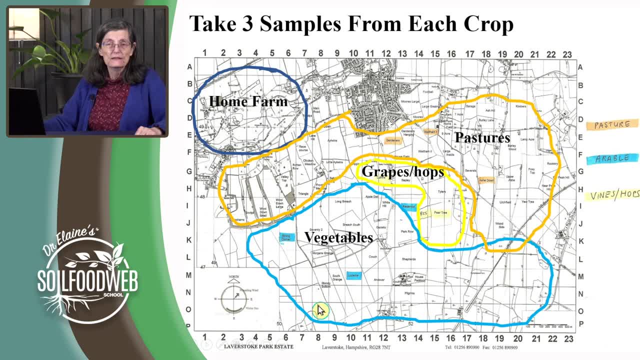 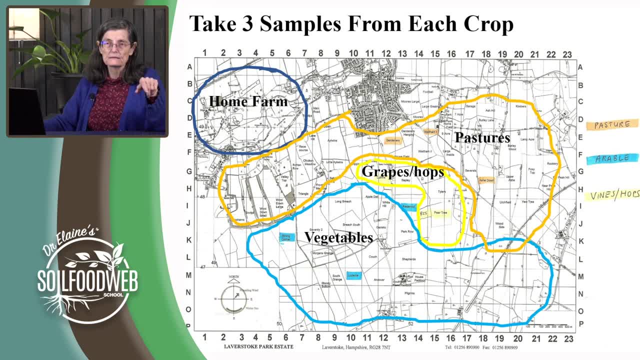 fields so you find out what's missing, what is out of whack, why don't you have the fertility that you require? so make certain that you're getting a good representative sample out of any of these fields and we go into that discussion in depth in the classes that we teach you. there's lots. 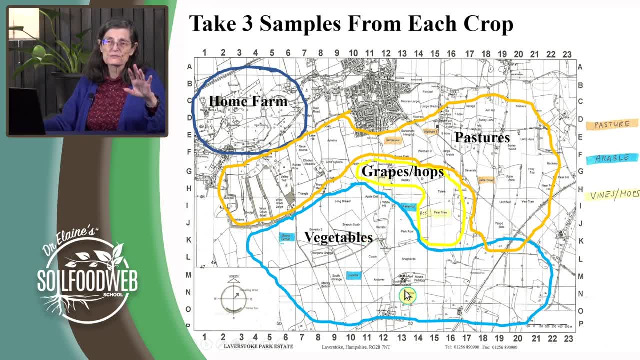 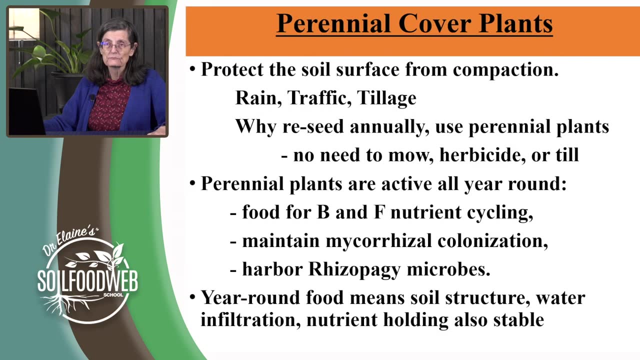 of things to be considered. lots of different ways of presenting this, so we'd want to have you for long enough that you can get a good comprehension of how to measure in a statistically reasonable fashion. cover plants, so protect the soil surface from compaction. you want to make sure that you have something in the way so that the drop 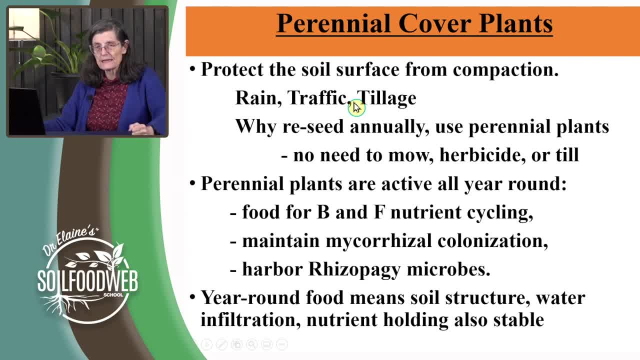 of rainfall are not causing damage deeper into your soil. the damage doesn't usually occur on the surface. when you're talking about raindrops, they're being. the energy is being transferred down to about five centimeters depth in the soil. that's where your compaction layer is going to. 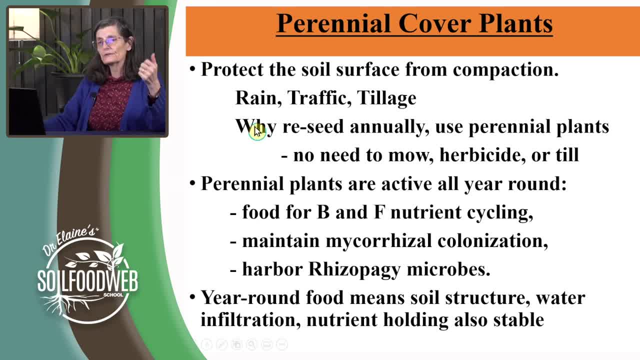 form. so be out there with a penetrometer and make certain that you figure out how far down that compaction layered is. so when 만약 kiorarit by the удобkatnüber desudoại man der wei dashi has happened, if you don't protect the surface of your soil, perennial plants. 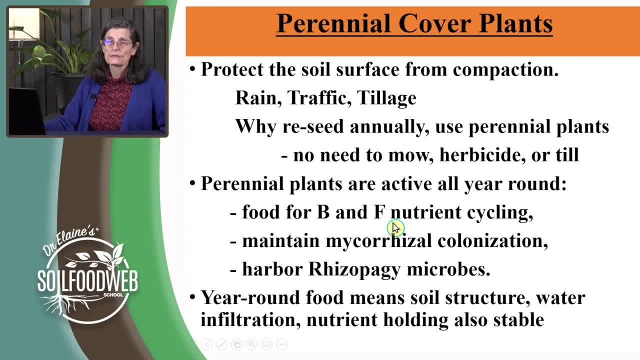 are going to be active all year round. you couldn't ask for better. you want to think about perennial plants are all going to be slightly woody or very woody and so fungal to bacterial ratios it should be pretty well equal fungi to bacteria or a bit more fungal. so the food that the perennial plants can be. 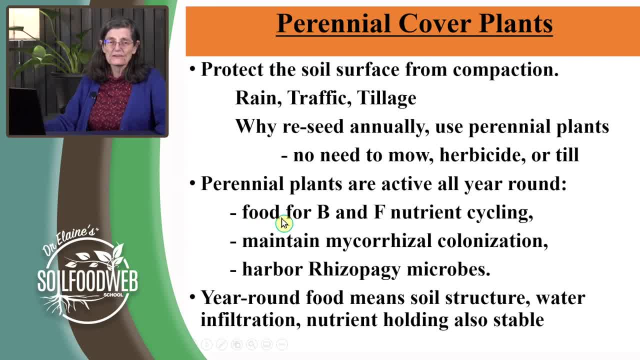 offering to your biology in the soil is going to have: make certain that the bacteria and fungi in your soil are going to be growing all through the growing season, putting away nutrients, making certain that you've got structure in your soil- all the benefits that we've talked about. you maintain the mycorrhizal colonization. if you till out, if you know board, plow everything, you just lost all your mycorrhizal colonization and now you've got to start over every year. you've got to start over reestablishing that mycorrhizal. colonization in the root system. it takes your plants approximately two months to establish mycorrhizal colonization. so if you're tilling your soil and you're wiping out your mycorrhizae, think about your next crop. you put the seed in and it's gonna take a while for that root system to start growing and 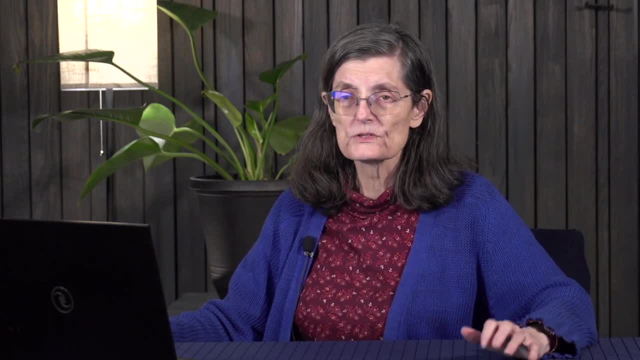 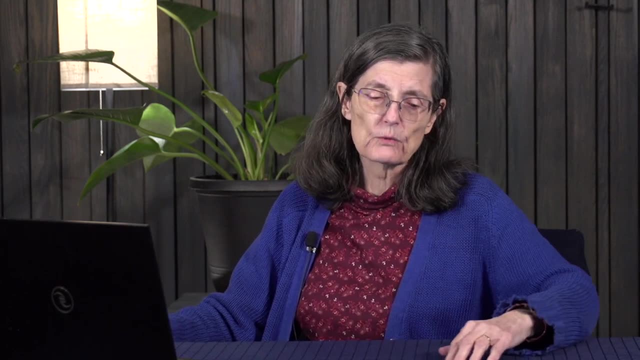 for those mycorrhizal spoors to go. oh, look at that, there's some roots around here. you're already in a month down the line. it takes another month for that mycorrhizal colonization to really form and start getting the quantity of 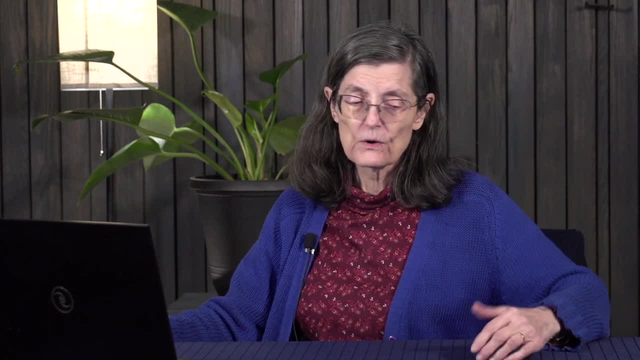 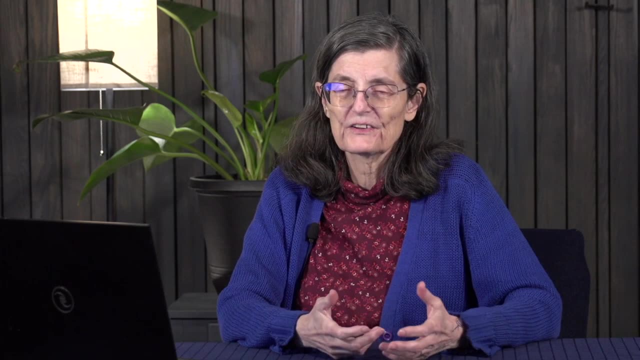 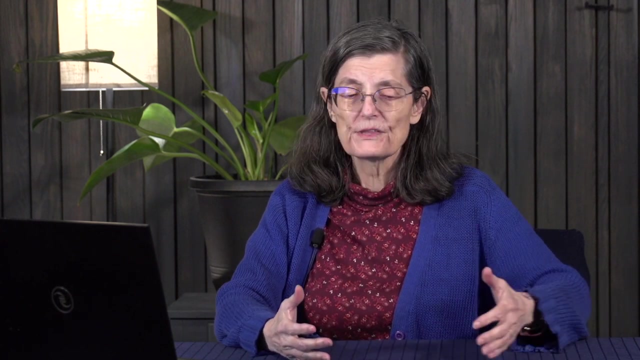 nutrients that your plan requires. so you have cropped it. only rose for six weeks. you're never going to get the benefit that you need. you need mycorrhizal root systems. they're already colonized so that the day your plant germinates and starts to grow. it's starting to get connected into the mycorrhizal system below ground, where all of the plants in that field are going to be healthy or without mycorrhizal fungi. all of them are going to be growing poorly. they're sick, they're unhappy, they're unhealthy and you're not. 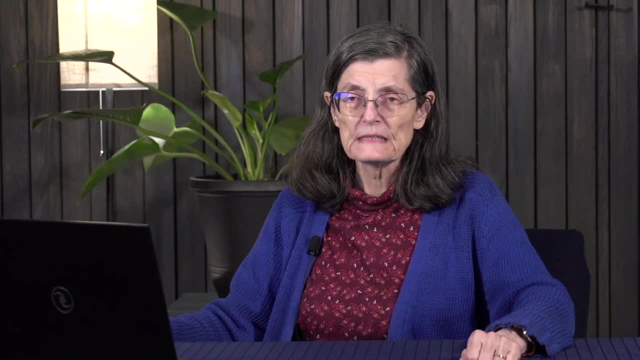 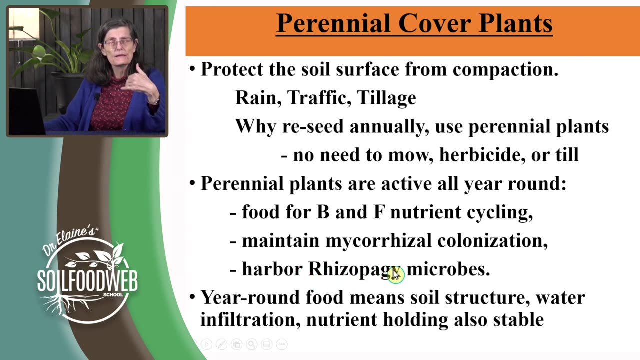 going to get the nutrients that you want. now we talk about rhizophagy and so another one of the new, the, the newer way that we've recognized nutrients are getting into the plants. so you know you're going to have to come and work with us a little bit. take our classes if you want. 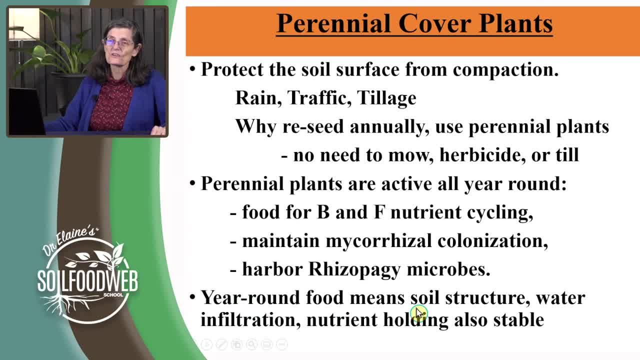 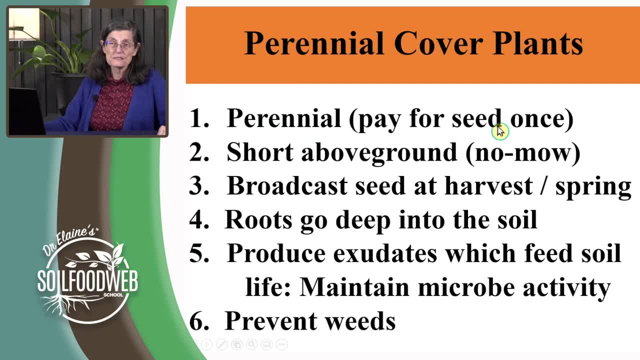 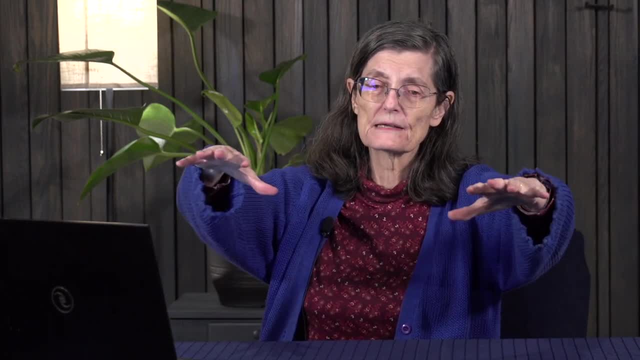 to get the newest, latest and greatest. so just what are the benefits of a perennial cover plant? you only pay for the seed once and then don't take the perennial plants out. you know you might put them in strips that are near the, the, the aisles where you know you're driving equipment. 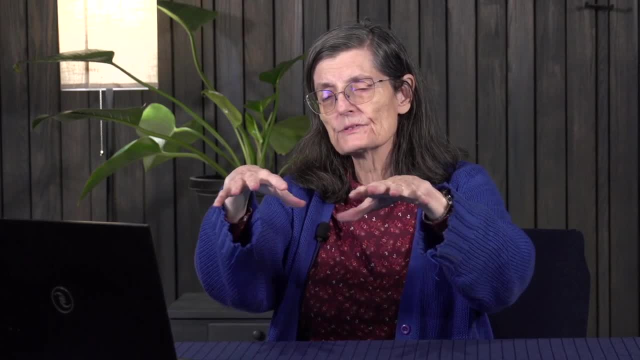 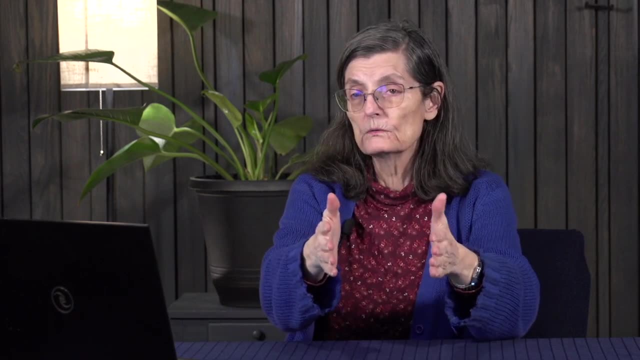 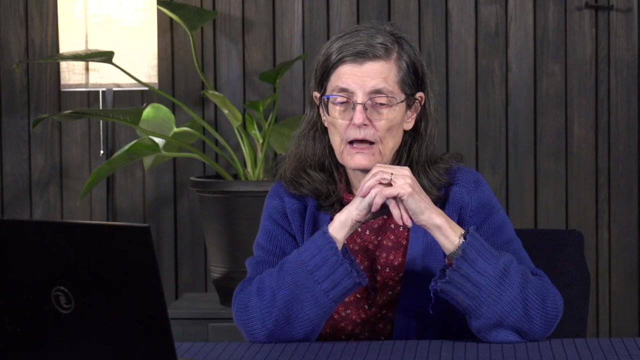 up and down, or people are walking up and down or maybe up onto the bank. where you've got your crops plants growing, leave a wide enough furrow so that none of the cover plants grow up and over your crop plant. you got to watch out for that when you're dealing with clover. 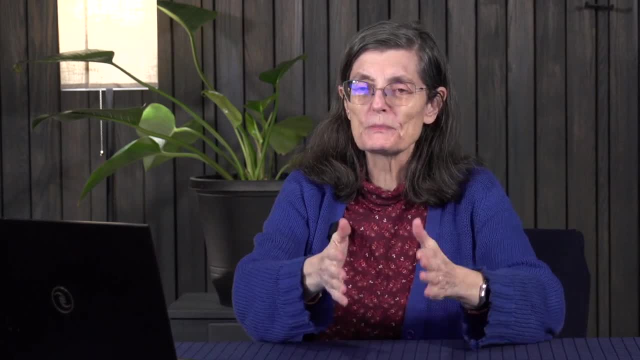 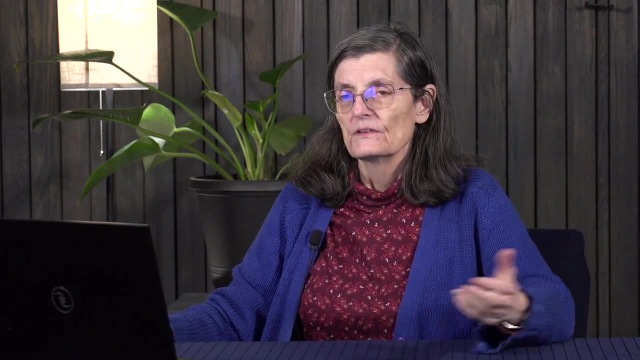 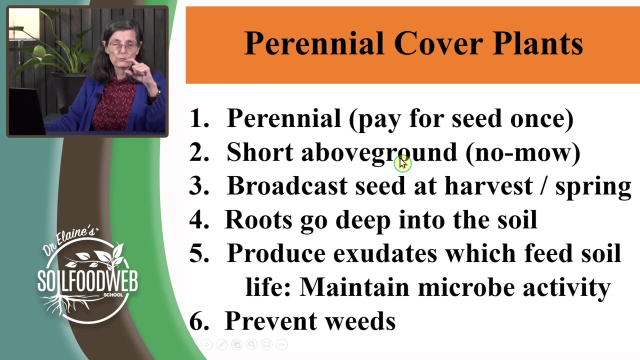 so a wide enough disturbance, but just that you know six inches of disturbance or eight inches of disturbance. we want to have short, low growing cover plants. you know one to three inches so you don't ever have to mow, you don't have to worry about some vermin is getting into your fields and girdling your plants, so that surprise. 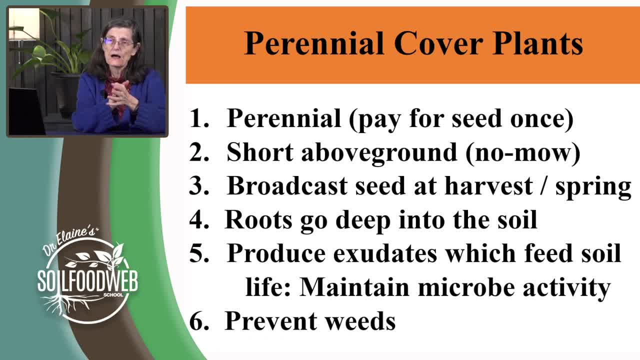 you don't have anything growing. you want to let the predatory birds get in and deal with those pests, and this is the part where the plants are growing. so don't be growing a lot of really tall plant material. you don't need to do that. broadcast seed at harvest for the perennial cover plants you. 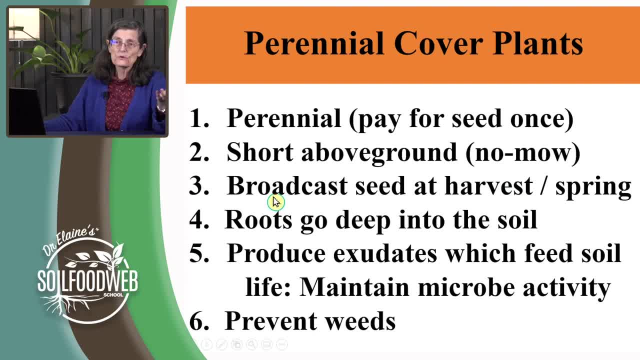 only have to do that once, and then those plants should be surviving for the next 100 years, 200 years. well, you know, you lost some because you know a cold snap that some of your perennial plants couldn't tolerate. so you broadcast seed at harvest and in the spring the roots go deep into. 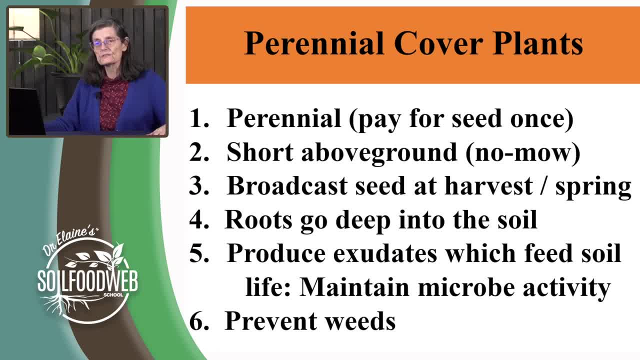 the soil. so they're bringing foods for those microorganisms deep down in the soil. they're bringing those food to feed those things that are building structure to hold water deeper in your soil. you want to produce exudates which feed the soil life. you want exudates produced. 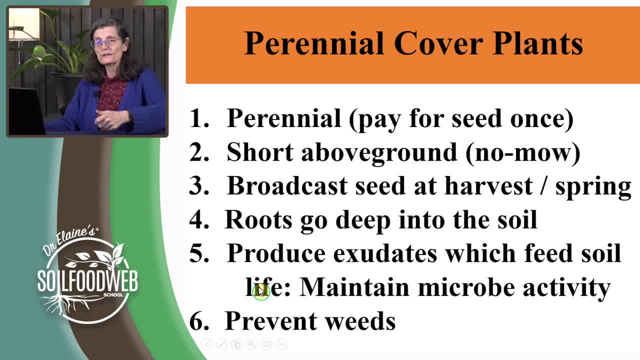 by those perennial plants that are going to go tell the bacteria and the fungi what they need to do to make sure certain that that perennial plant is getting all the nutrients that it needs. so you have a non-stop, never-ending way of preventing weeds. so all the benefits that you can get. just an example: 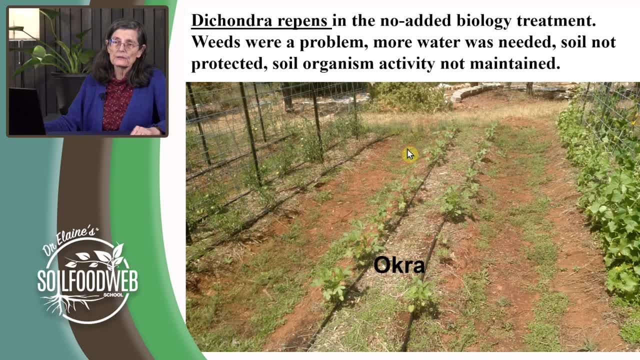 here's a system where we put in dicondor weapons and this is the control plot where we're looking at no additions of biology of any kind. so looking at your tomatoes over here, you know this is the no added biology. treatment and weeds were a problem needed to be adding water all the time. soil is not protected. this 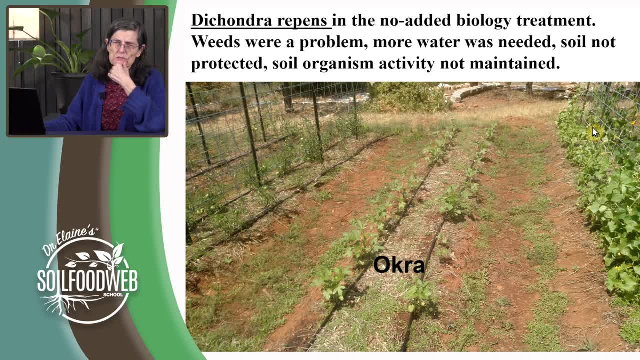 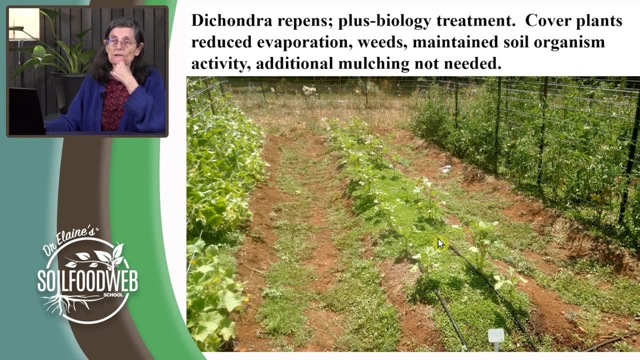 is okra in the middle. this is- i believe this was a squash. it's hard to tell. from this picture now, where we added biology, you can see that the deconder is growing much better. less of the system is bare. now look at this row where no walking and no traffic. 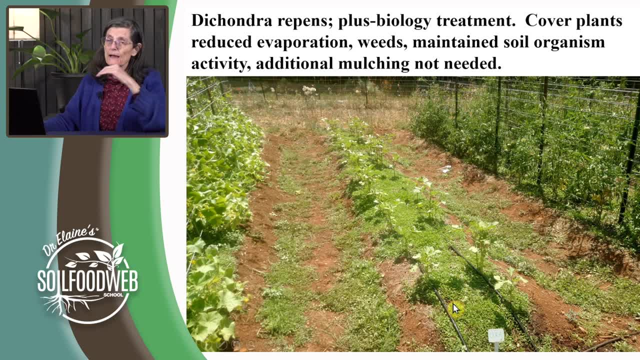 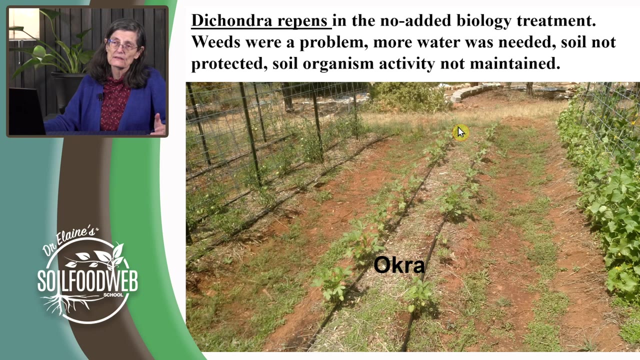 was allowed because it's in the middle of the bed, completely blanketed by the cover plant, the perennial cover plant, and all of these okra. okra are in bloom. On the same day this picture was taken and there's just a few of the plants that have survived, actually, and the number of flowers is. 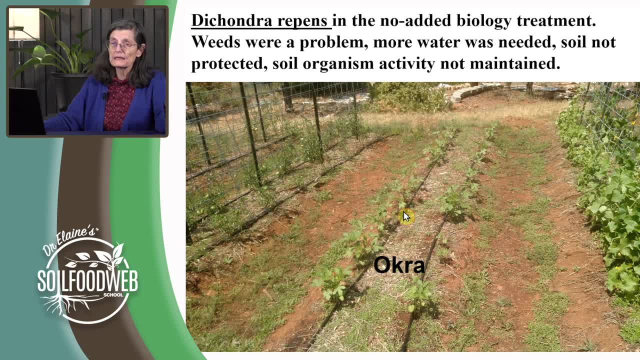 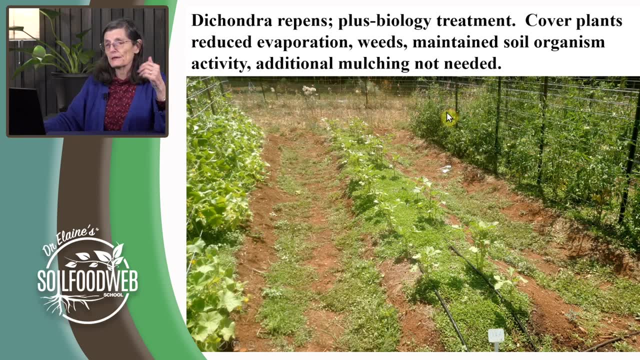 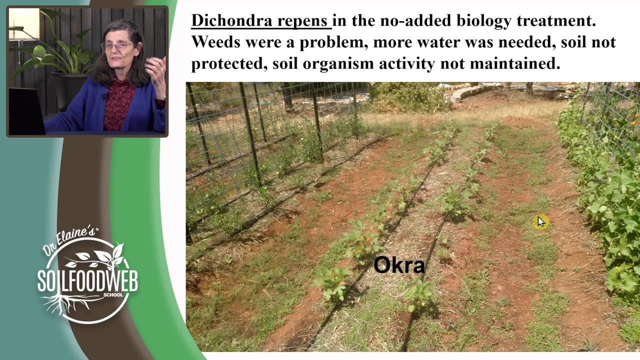 not as far along or as many as in the system, where we have the cover plants and the additional biology. Look at those tomatoes. You want these tomatoes, or do you want those tomatoes? So I think it's pretty hands-down. biology helps you and 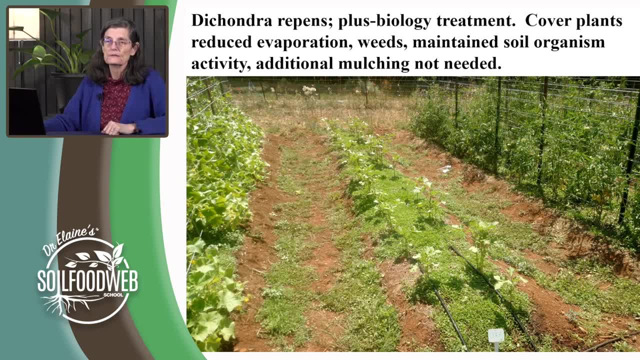 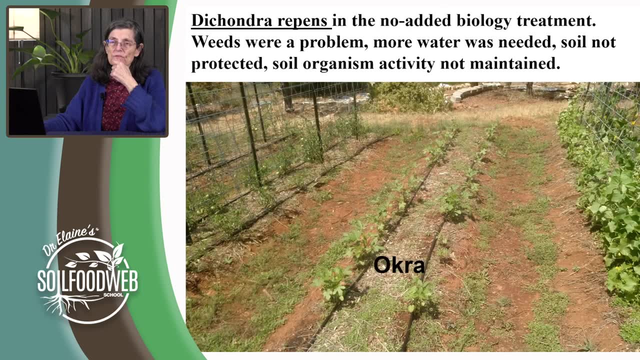 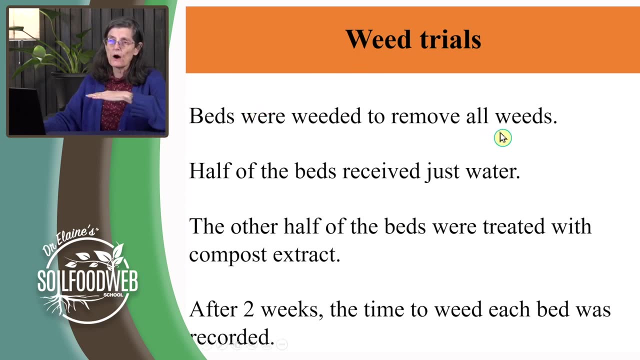 the cover plants also help you. So huge, significant strides forward and a much higher yield. So the next is a weed trial, where the bed were weeded to begin with to remove all the weeds, and you know the weed bank and all of these plots were at the same place when we started out. so we weeded. 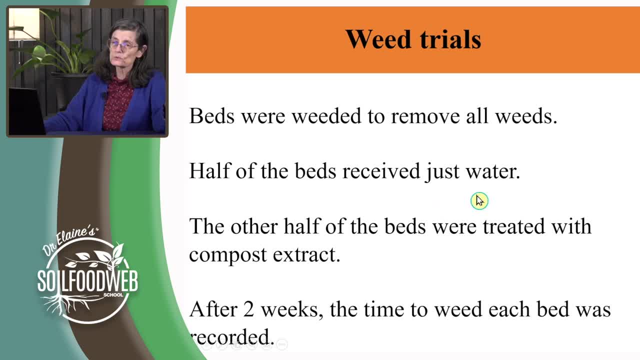 those plots. half of the beds then got just water. the other half of the beds were treated with a compost extract after two weeks. so we didn't pull any weed out. it was hard to prevent me from going out and starting to weed after two weeks. the time to weed each bed was recorded, so we cleared all of the bed of. 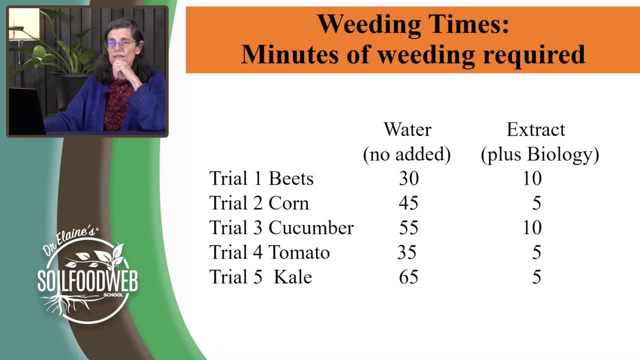 all of the weeds in each instance and these are the data, the minutes that it took to weed those plots. so the beets: 30 minutes where we just add water, versus where we had the biology: 10 minutes. I don't know how many we how many minutes. 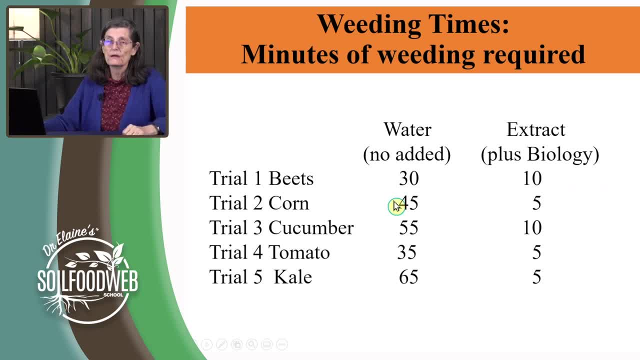 do you want to be weeding? and I want to keep it down to a dull roar. okay, corn, 45 minutes to weed that, versus five where we had the biology. what does that tell you? all of them? over here, almost all of the nitrogen was nitrate over. 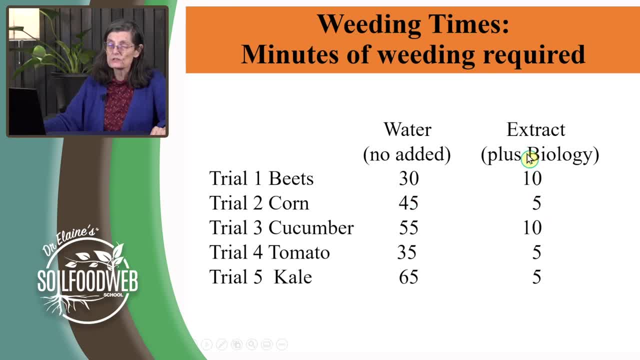 here. not much of the nitrogen was nitrate. it was mostly ammonium and you can see the benefit. so all of these things factor into the benefit that you're going to get cucumber 55 minutes versus 10, 35 minutes versus 565 minutes versus 5. so 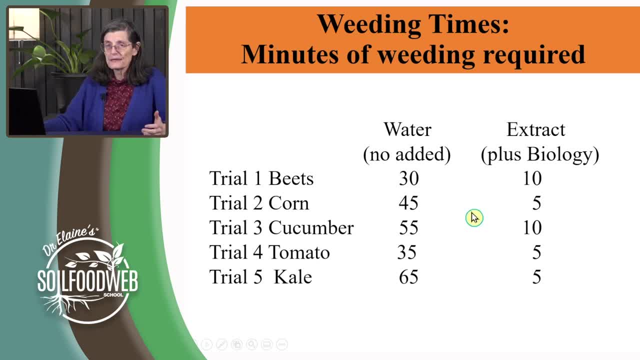 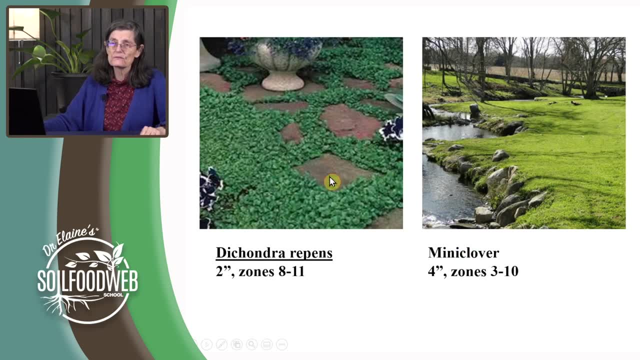 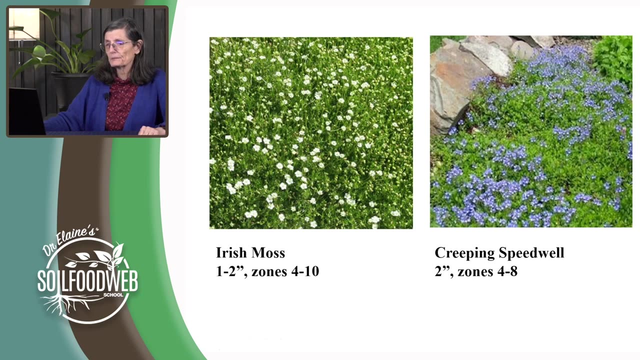 get the cover plants out there and make sure to get your biology out there so you can get these kinds of benefits. so, dichondra repens, and this is mini clover- we've got lots and lots of different kinds of cover plants that you can use. 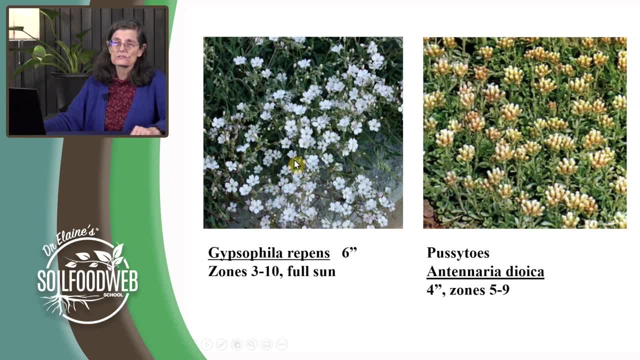 you can already pick one if you're a plant here like that, right there, and just some pictures to show you what they look like. always put seed in several pots so you know what these things look like as they're popping up out of the soil and you don't have somebody that goes and weeds your perennial cover. 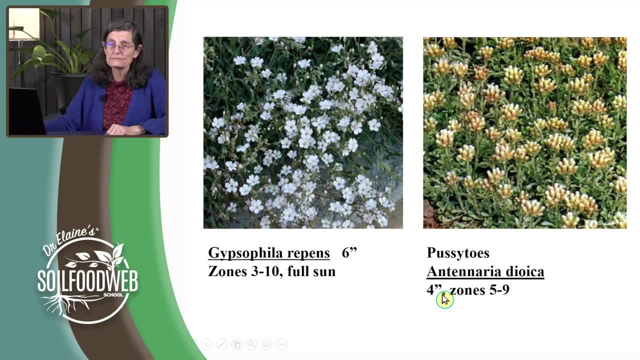 plants. so you know different zones: 3 to 10, 45 to nine, you know. so pick what's, you know, full Sun, the zones that they can grow in the typical height that they get. you know, six inches here might be getting a little high. four inches, that's pretty good, like this one to two. 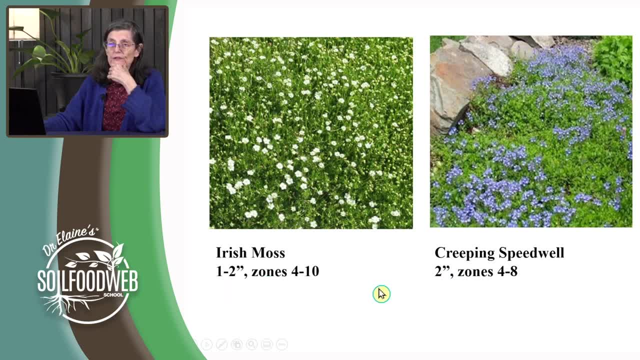 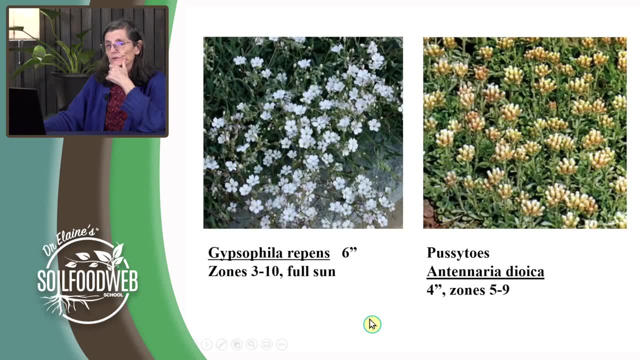 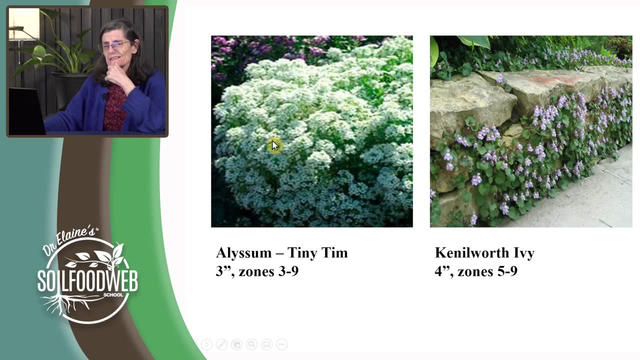 inches, two inches, so very good, and the speed. well, is quite woody, being some of these farms, client plants can be quite woody in character, so perfect for what we want to do. Alyssum: one of the things with the Alyssum that we notice is that when we put it into a really good fungal to bacterial 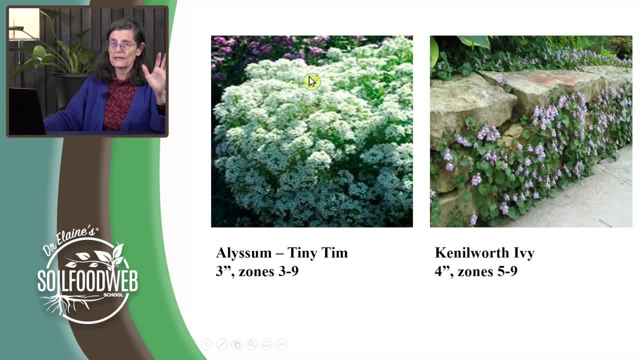 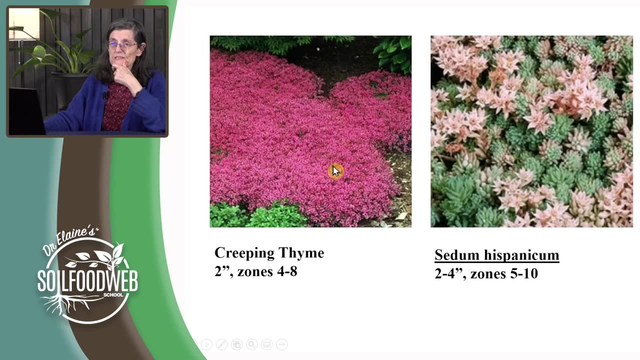 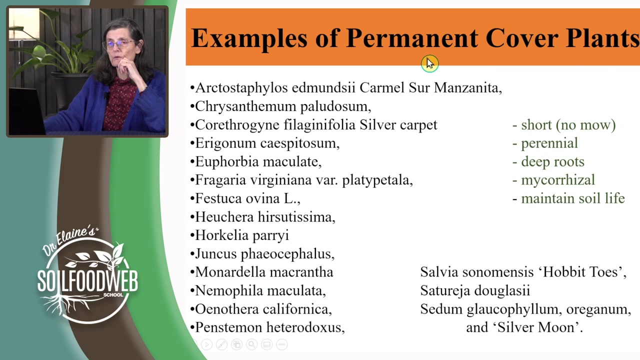 biomass ratio. the flowers just take off and they do not remain two inches, they're going to be up five or six inches, which maybe puts them out of the. you know the real cover plant system, so you be testing your own cover plants. we do have, you know, a list of men of quite a few of the cover. 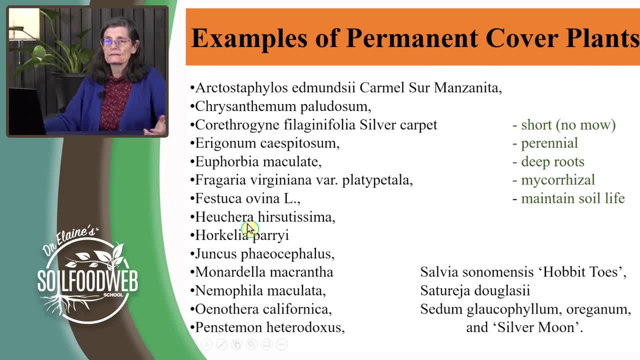 plants that we've have been testing and what you would want to do is go to some botanist or nursery where they like to understand and know the different species of- and we always want these native plants or indigenous plants- and find out sources of the seed for them. use one of the other species of these perennial plants. don't go along and just say 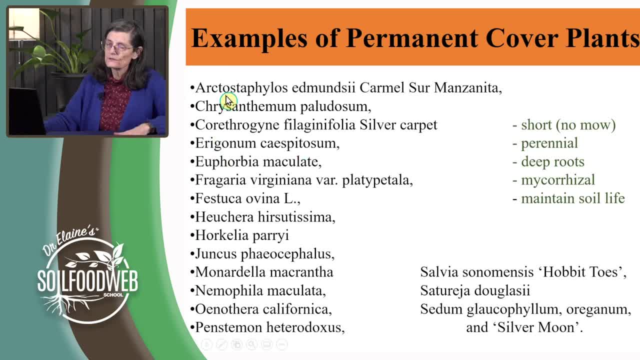 oh well, this is good, and that's good, and that's good. go to that botanist, go to that nursery and find out what is the indigenous species of euphorbia or herkelia juncus. well for you, then we have. the first, how to check if the plant is двигating in this area. well, first, if you're looking to, 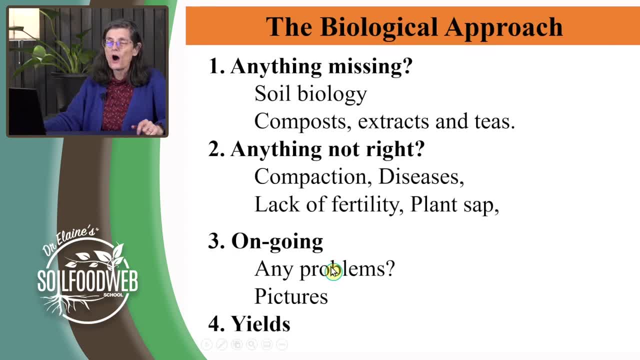 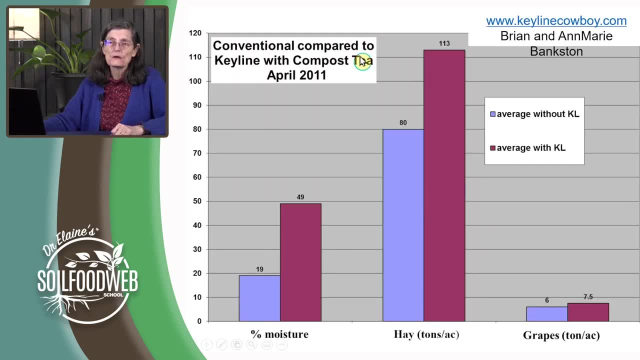 get the plant that's dropped on the ground and then we start testing the plant. you'll see that this is the first time that is working, and then we start testing it and the only difference is that we don't want to get it into the ground. if you're looking at the lower part of the world in 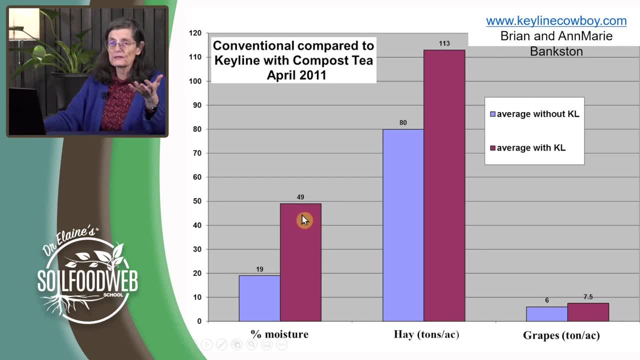 your bio region. that's what you want to get into the ground. just check and make sure it still stays a short growing plant, long on the roots, short above ground. so just to give you some examples, the only difference between the control and the treatment is that, I think, only apply the 3 applications of the compost. tea was applied and look at the increases in yields. so from 19% sharp 1% seed size, 2,500t 100% transplant. 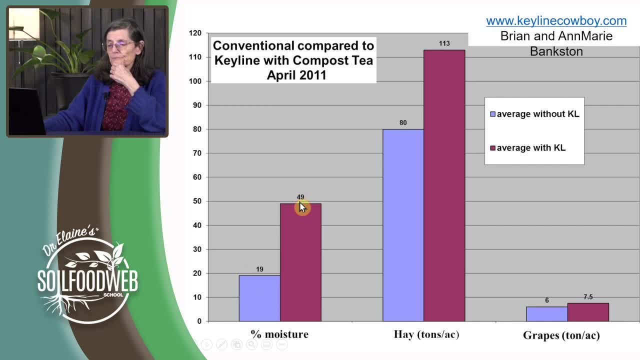 to 49 moisture. sorry, this is not a plant yield, this is percent moisture. are you holding water in the soil beyond shadow of a doubt because of the biology? here we have the hay that was produced in that field. so the difference between 80 and 113 just by applying compost tea a couple of times in grapevines. this is 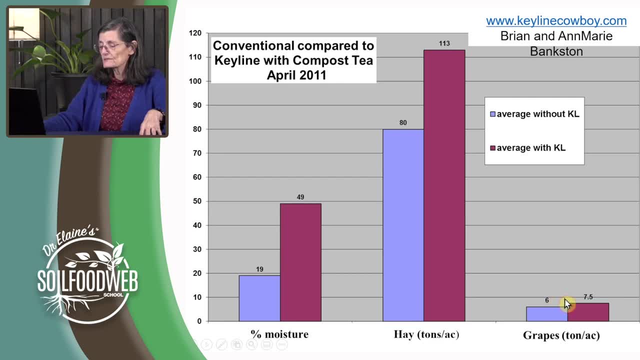 just the grapes that were picked, and so six tons versus 7.5, that's quite an increase in yield for grapes. so this was in Tennessee, the the work, and if you're interested you can get hold of Brian and see what he's up to these days. say hey. 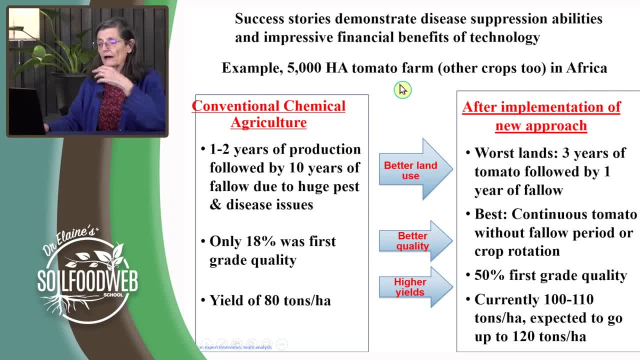 say hello to him. for me, we're coming out of Africa where we're looking at conventional chemical agriculture: one to two years of production, followed by 10 years of fallow before you could get another tomato crop into the system and actually have it live the roof eating nematodes. 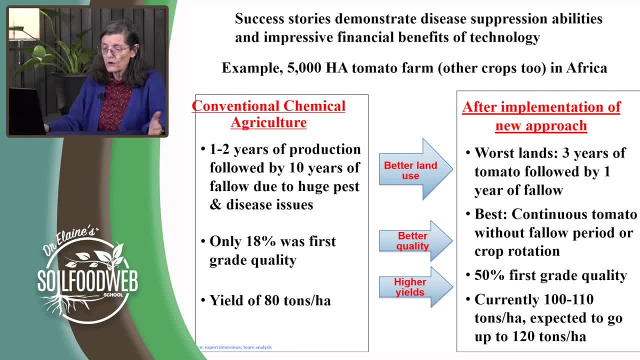 were out of control here. only 18% of their tomatoes were top quality. that's not enough. you want 50% or better. a yield of 80 tons per hectare- not enough. after we implemented in the very first year the worst places, they got three years of potato tomato production, followed by 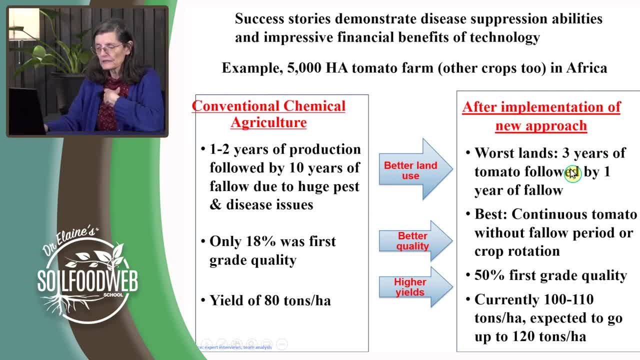 one year of fallow, they went back in. they thought they'd test their luck. and now those, even the worst areas, are tomato, tomato, tomato, tomato, tomato tomato and probably will stay. no reason to rotate if you're getting the biology back into the system. they are doing all the work. 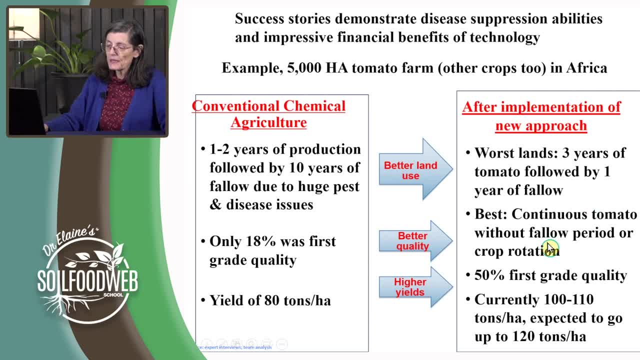 your plant doesn't have to do the work. continuous tomato throughout the fallow period, no crop rotation, 50%, first-grade quality. they're up to. I think they're beyond 120 tons per hectare, but I haven't talked to them in a few years. so 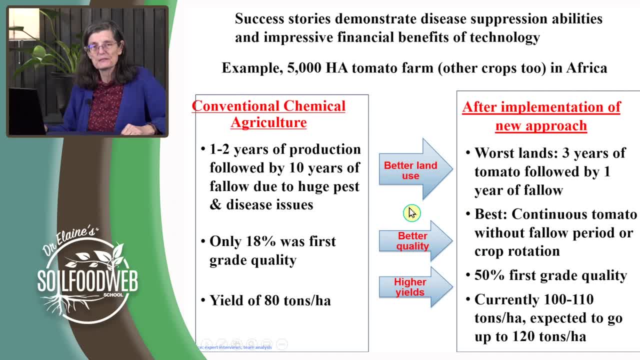 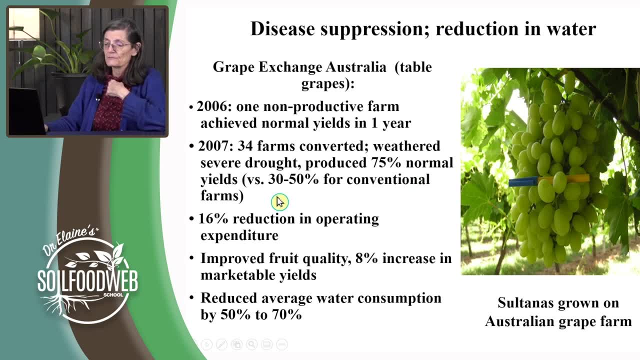 again ZZ2. you might be interested in getting hold of them and seeing what they're up to. disease reduction was reduced. they were in the middle of a drought, so they gave us this one. the grape exchange. Australia gave us this one farm that had never produced grapes. 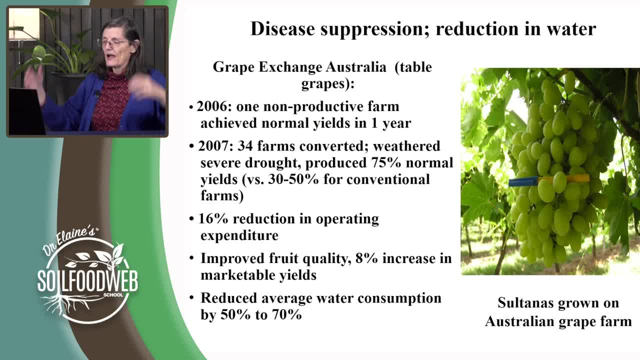 before and they just kind of figured what's. how could we lose if we can, if they can go ahead and get these grape vines to produce, why not let them try, and so in 2017, because of the results we had: all of their farms were out of control. 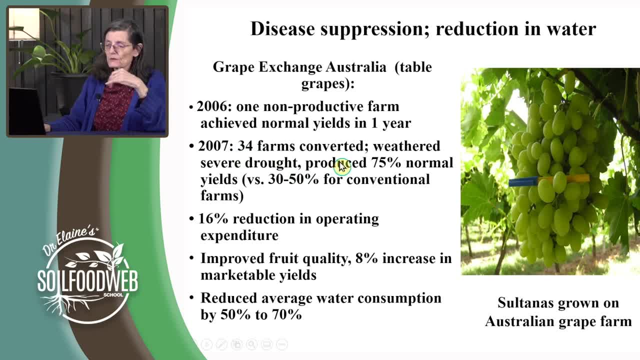 all 40. 34 of their farms were converted into the biological approach. yeah, they didn't get the normal production, but remember we're in the middle of a drought, and a drought that has been around for 40 years. so 16% reduction in the operating expenditure. improved fruit quality: 8% increase in marketable yields. 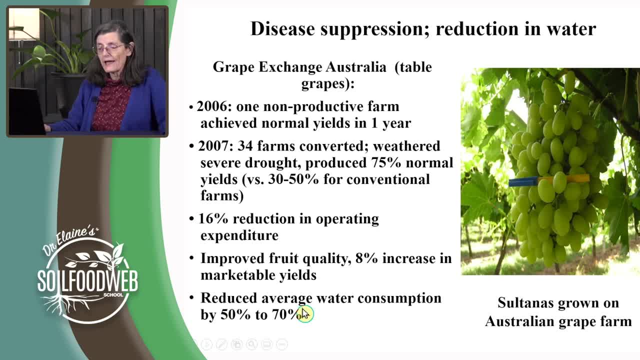 that's a massive amount of money, reduced average water consumption by 50 to 70%. and that was the real trick. when there was rain, slight as it might have been, all of that water infiltrated into the soil and held that water in the soil. they did not have to water their vines. 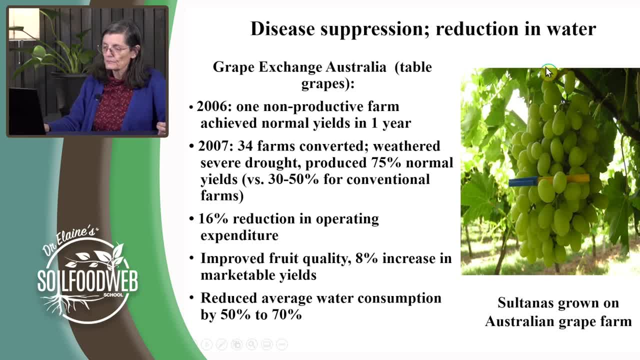 and yet look at those the results. one of the few places that to provide grapes into the supermarkets and when you're the only group of people with table grapes to sell into that market, you can get top dollar and so they made a huge amount of money. yeah, it was still 75 percent of the normal yields. 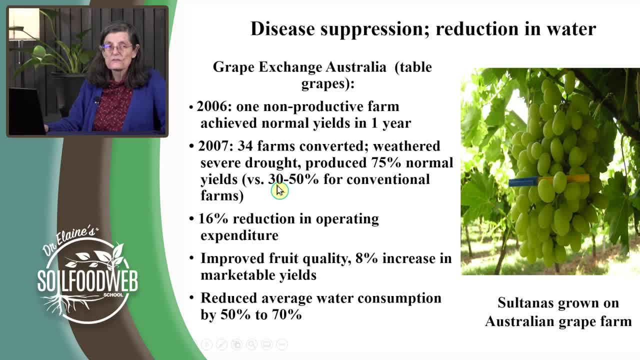 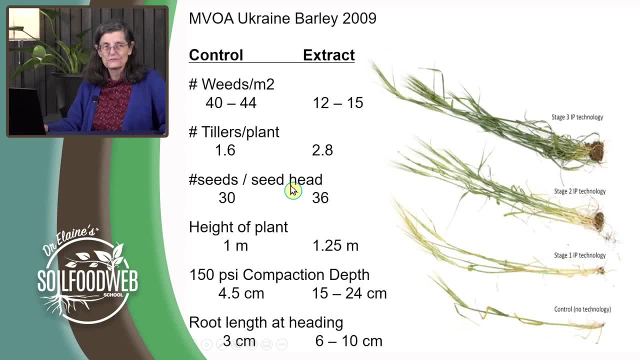 but the conventional systems 30, 50 of the normal yields. so what do you want? normal or biological? this is working with ukraine barley in the ukraine. this is with maharishi university in iowa, the. these are the results of, if you just compare all three of these practices, 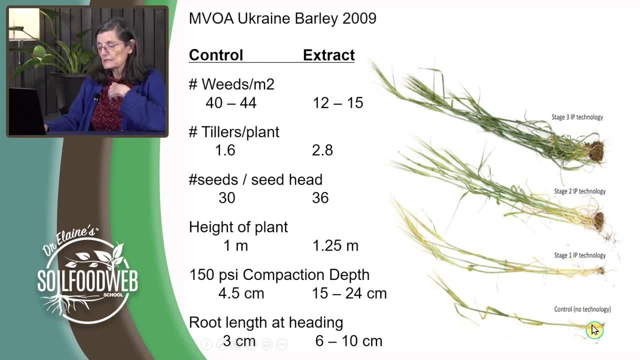 the control treatment. I want to go just a little deeper here. we pulled out just one seed. these are the tillers. off of one seed you can see the tillers increase. not quite a bit. and there's the tillers increase a lot with this one seed. this was in the control. so no technology, no life put back into the. soil. one seed, one stock, one seed head at 30 seeds per seed head. when we treated the seed with compost extract and then planted it, we got three tillers on average three seed heads, and each seed head had 32 seeds in it, so huge increase in yield. 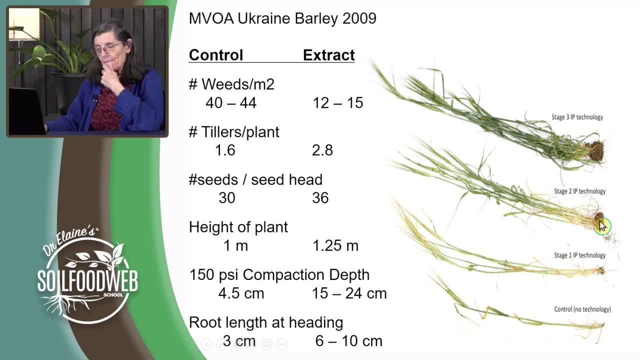 there. this is a single seed, but that seed was treated with compost extract before it was planted and then it got one application of compost tea once these tillers started growing, and so you can see how many more stocks so there's: gosh one, two, three, four, five, six, seven. now let's say seven tillers and each of. those had 34 seeds in that seed head. one seed was treated with compost, exit with was treated with biology on the seed and then two applications of composty we're looking at. I think this is 15 tillers, each tiller having a seed head and 36. 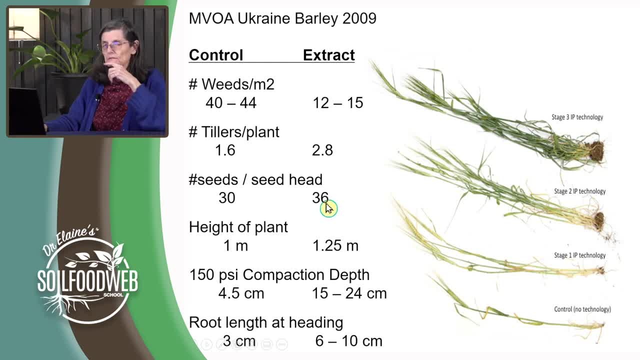 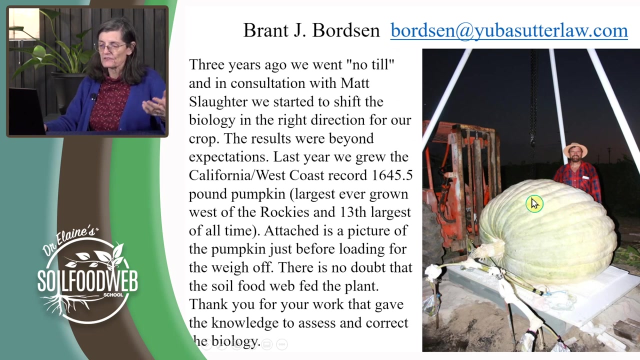 seeds per seed head and They were a little well, that's just you know. they were so proud of that Improvement. in the barley production We work with all kinds of people doing all kinds of crazy things. I love this one because They were no-till and so in consult, in consultation with one of our lamps. 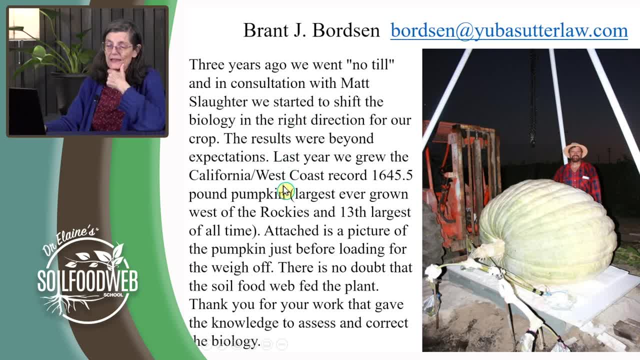 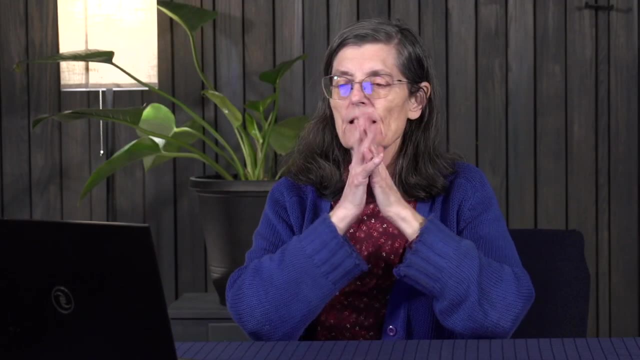 They shifted the biology in the right direction and they had the record for the biggest Pumpkin ever grown. So I don't think anybody's past that level yet. So They only could do this Because they had the biology in the soil. so some examples of the work that we've done and 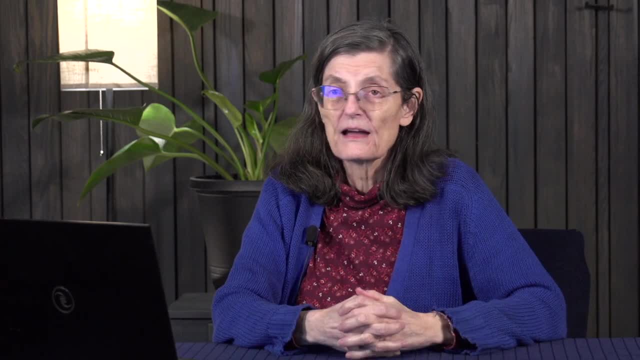 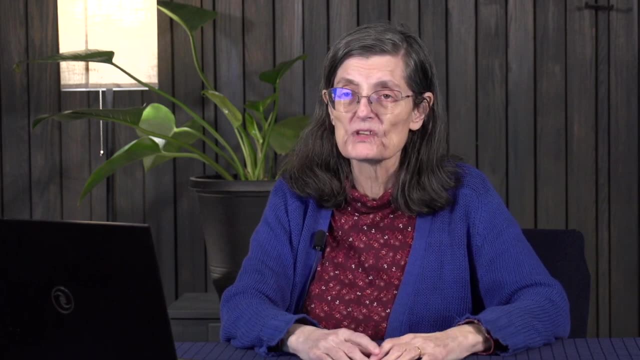 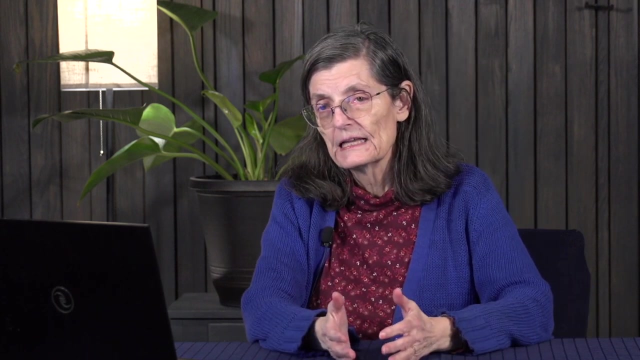 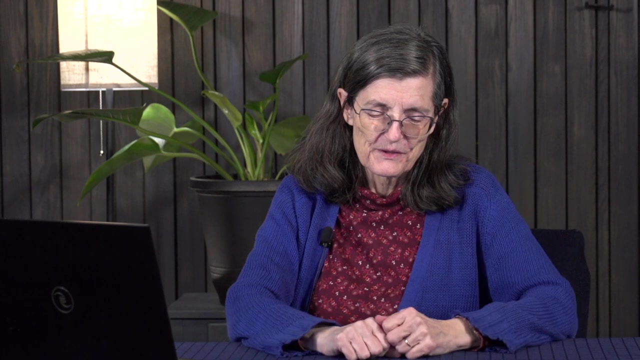 You know just a smattering. We have the school now coming along where all of the students to become consultants Have to do their own trial of converting dirt back into soil, And so we will be adding their certification process product and their certification Program into our website. so please go look at our website. 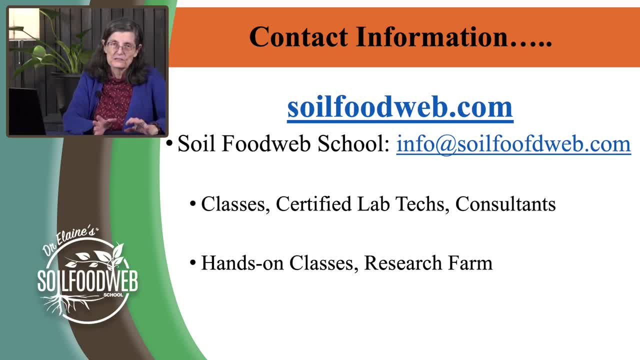 it's, You know, soil food web, comm or our. send a message to the soil food web, school info at soil food web, calm, And Then we are. we will have Some hands-on classes, We're hoping, at the research farm that we're going to be starting up this year. 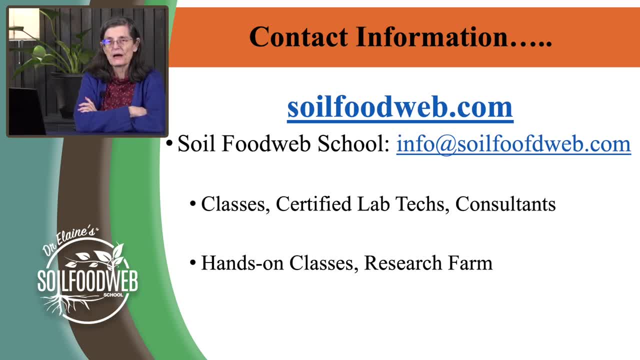 And please, you know, stop in and find out about our classes, Our foundation classes, where you get all the background information, where we train certified lab techs, if you like that part of Helping people get the right biology in their soil and know that they've got the best data possible. and 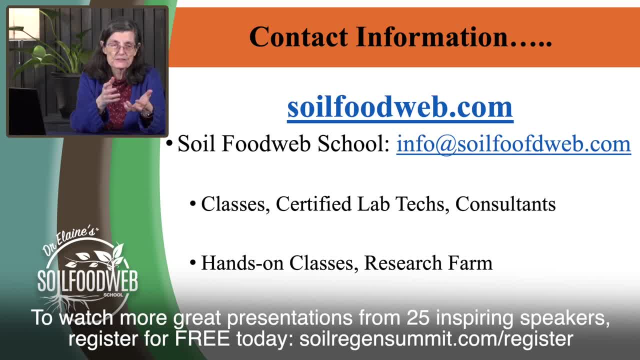 then the consultants, which have been trained as certified lab techs as well as Doing their time, and the students often call it: We're doing our soil PhD When we're doing these conversions of dirt to soil. So with that, thank you very much for paying attention. 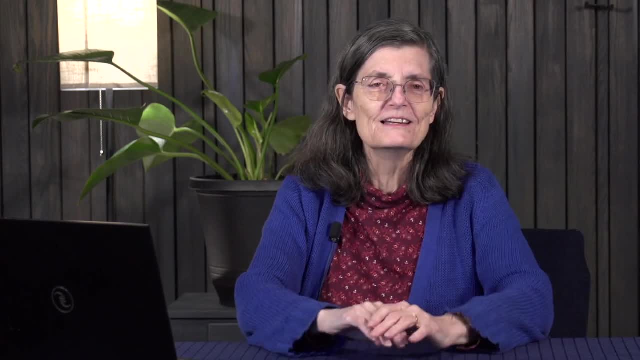 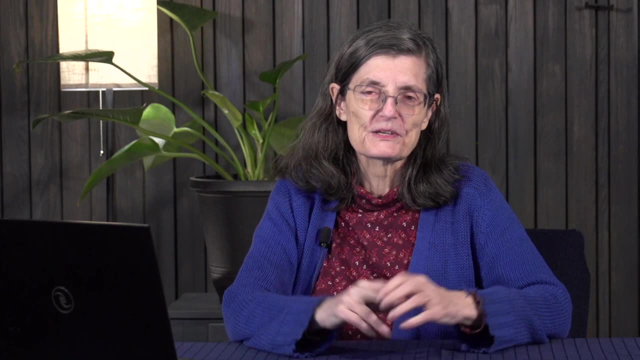 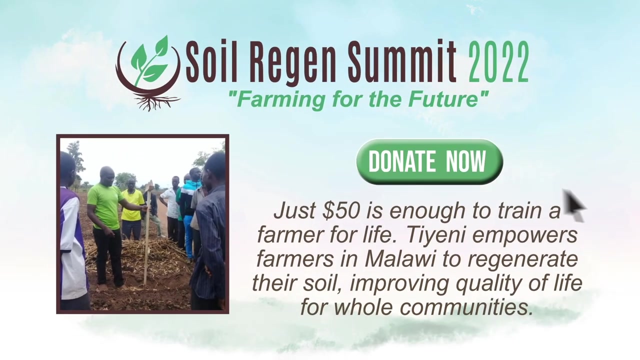 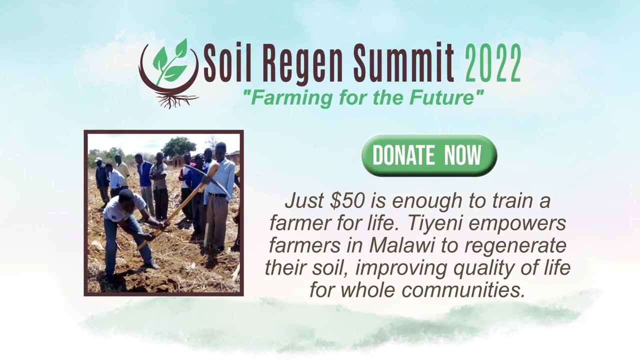 wish you all kinds of fun watching the rest of the The some soil summit presentations for the rest of today. thank you very much. Just $50 is enough to train a farmer for life. T&E empowers farmers in Malawi to regenerate their soil, improving quality of life for whole communities. 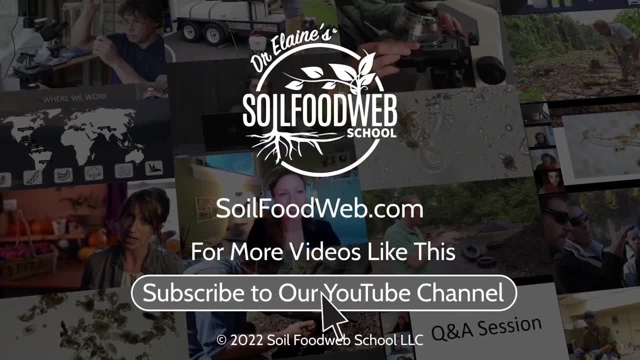 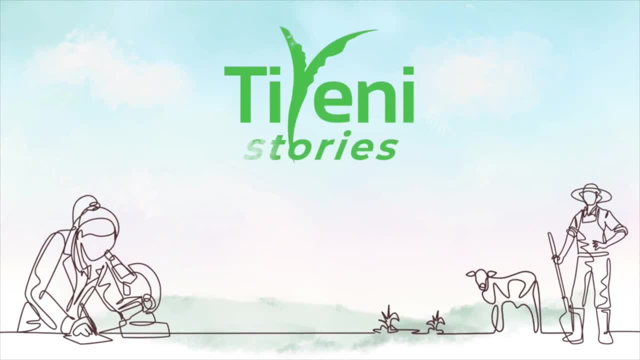 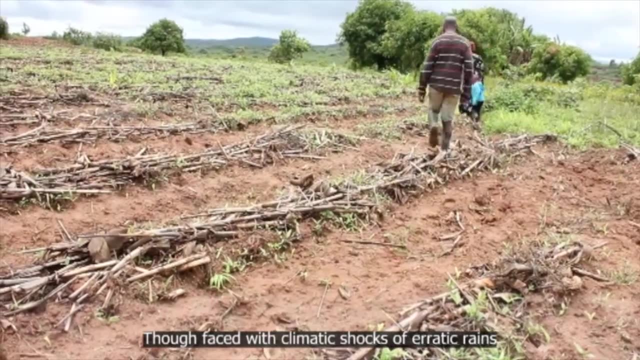 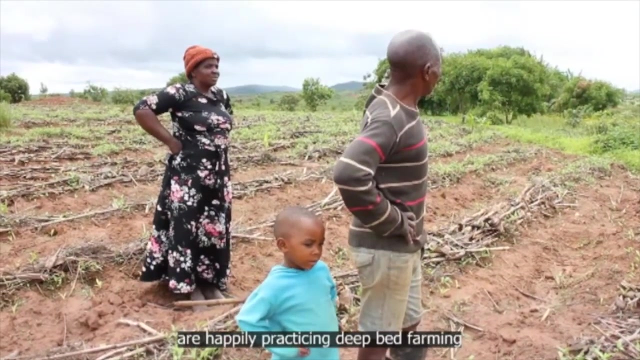 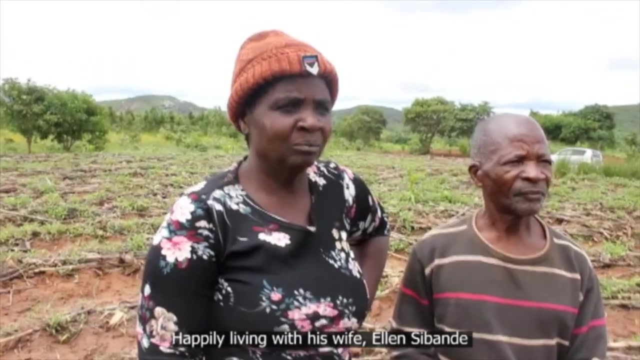 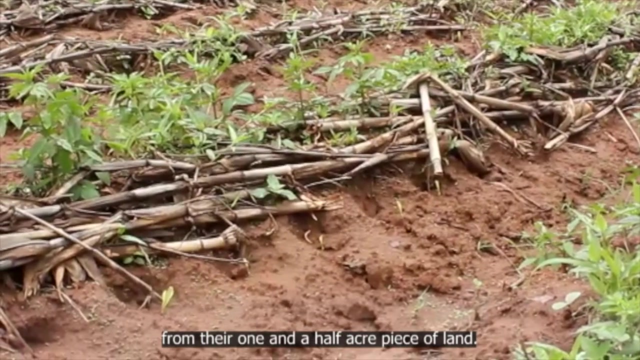 For more videos like this, subscribe to our YouTube channel. Though faced with climatic shocks of erratic lens, the family of Austin impound of Jivanga area And the MCC in EPA are happily practicing debate farming. their only hope of bumper yields. Happily living with his wife, Ellen's Randy, the couple have clearly transformed their lives. from their one-and-a-half acre piece of land. 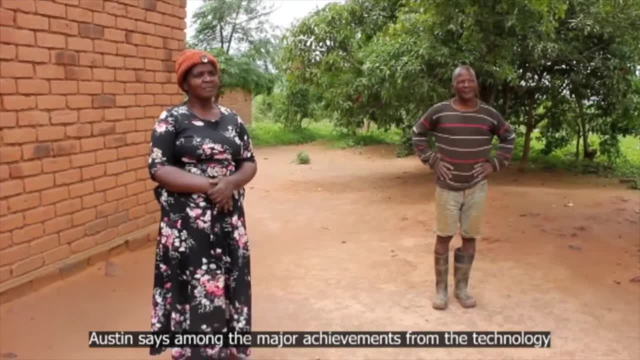 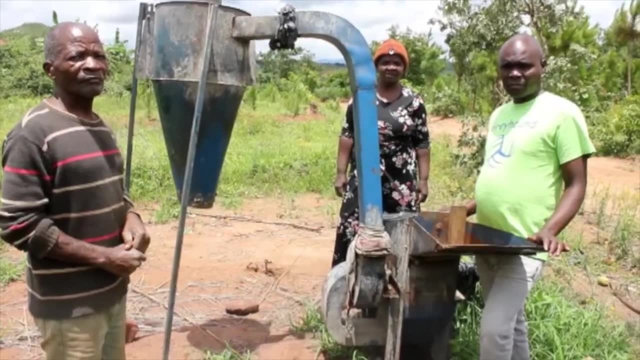 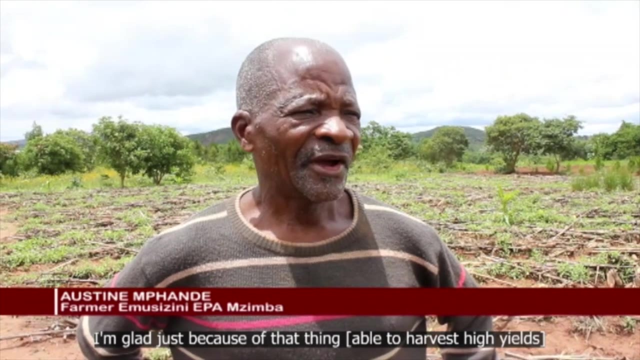 Austin says, among the major achievements from the technology, a big house, pigs and cows, including a maize meal, and We harvest more crops. So that is what always. I'm glad just to do that thing. He further says the work is very simple and a marriage strengthener. Before it was about the recent, that yours about the 20, but see how to get it. but now